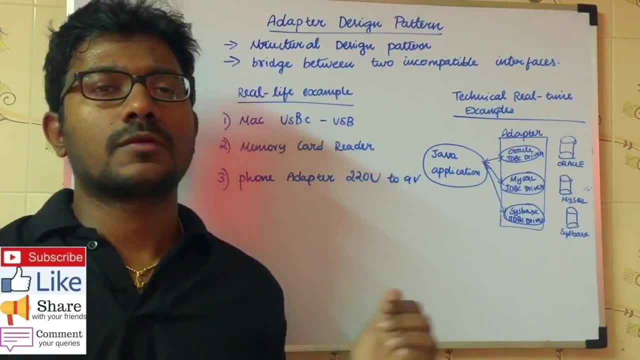 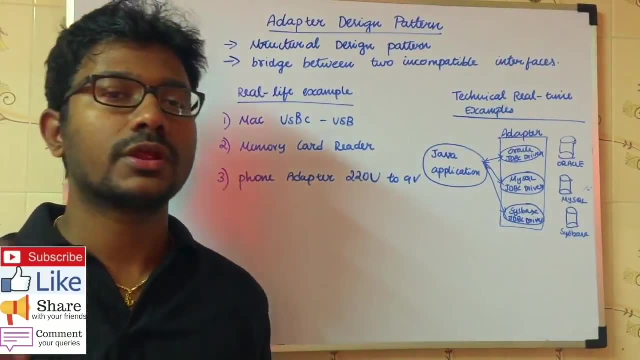 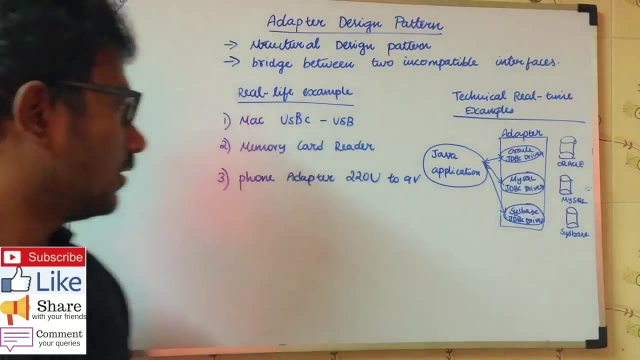 means at most of the laptops and pc there won't be any memory card reader in bit. so what you do is you will try to get a memory card reader for that and you will try to insert your memory card in that and you will try to connect in the usb port. this is one of the adapters and then is a. 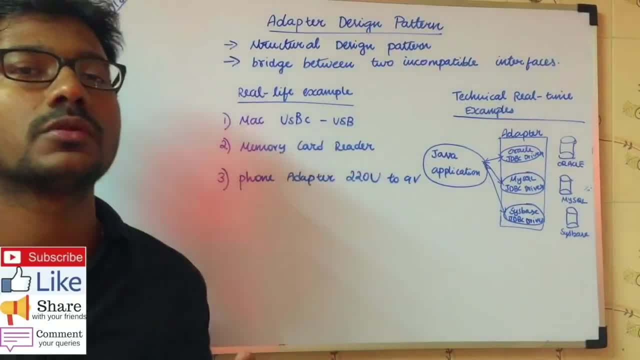 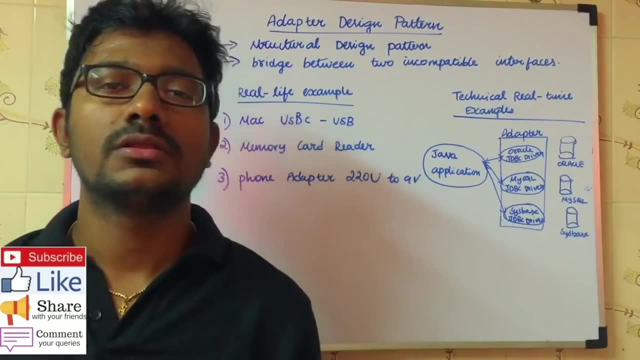 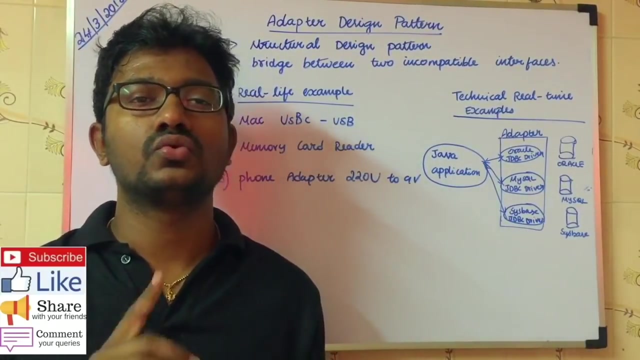 phone adapter. suppose, if you are trying to charge performance, what you do is you will try to insert the pin into a phone and you will try to put the adapter in this socket. that adapter, what it do is it will try to convert the 220 to 220 volts. so basically, in india, 220 volt is the power that we 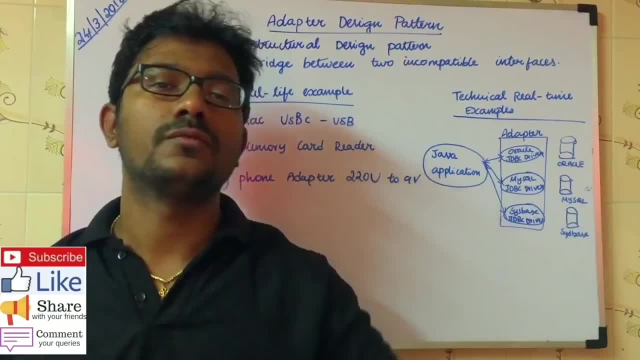 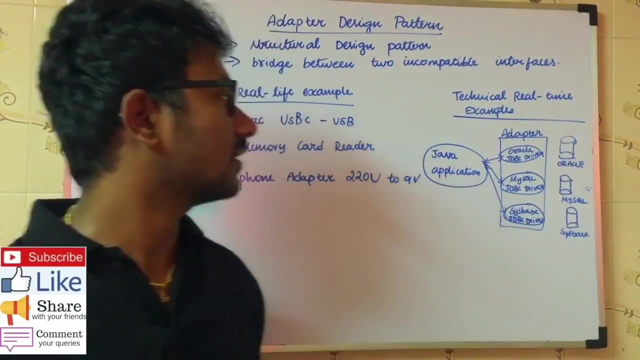 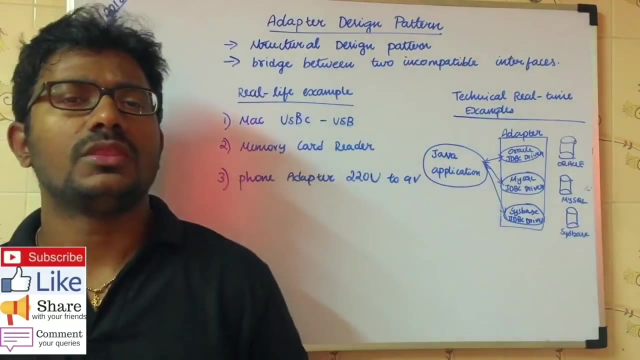 are getting for household purposes. so it will convert the 220 volt to 9 volt for phone applications, for phone usage. so this is the real time x real life example. these are the real life examples. we'll try to cover the technical real examples. if suppose, if you are using, if you suppose you are writing any java application. 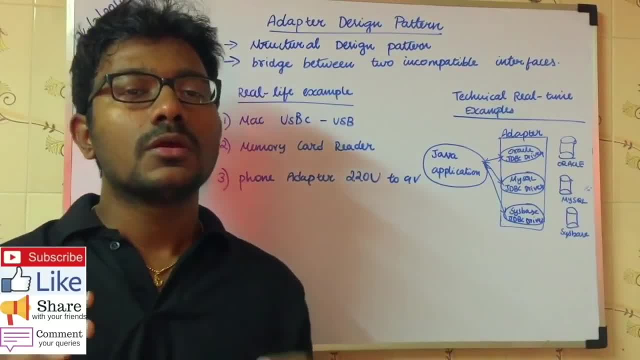 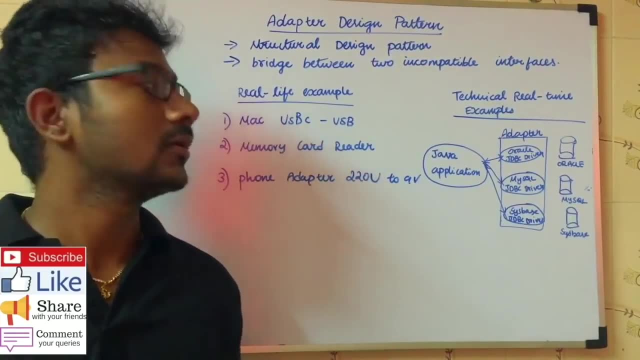 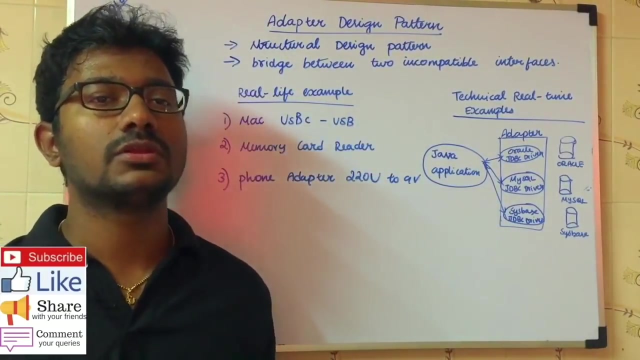 and that java application needs to connect with the database means for the people you write in java page they don't aware about the database that is behind. for example, it can be oracle, or it can mysql or it can be sysbase. based on time, the database may convert to the advanced. 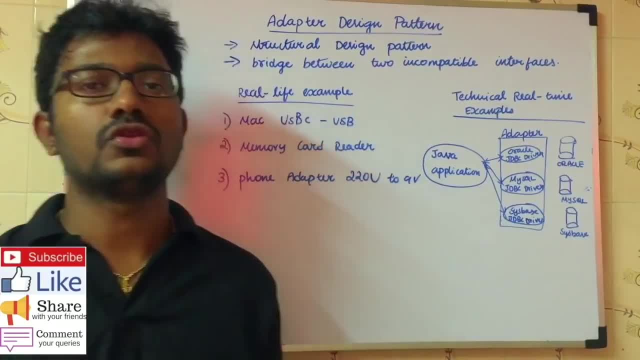 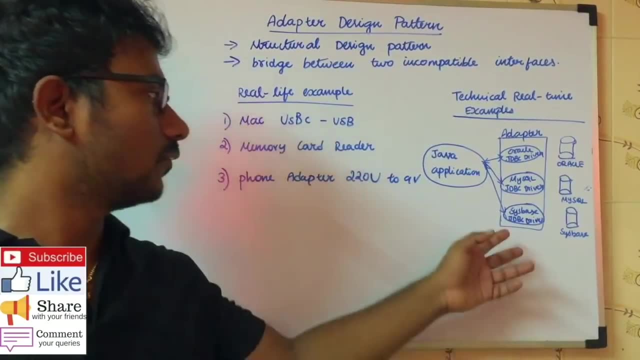 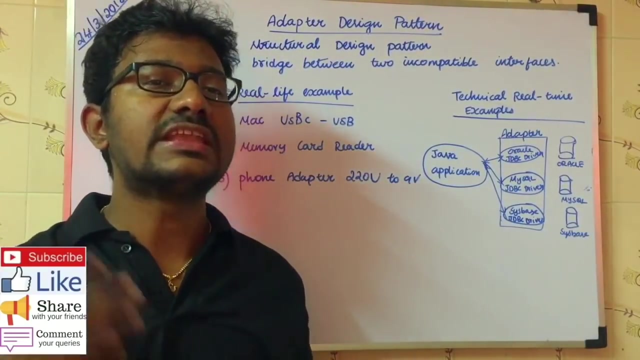 databases, for example. so if suppose if a new vendor is providing a better database means the people began, that would change that. uh, what to say that actual database thing? so we don't aware about the database that began running. you just need to write an application using some command. 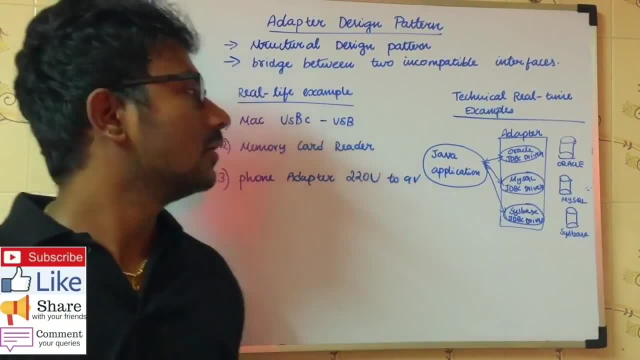 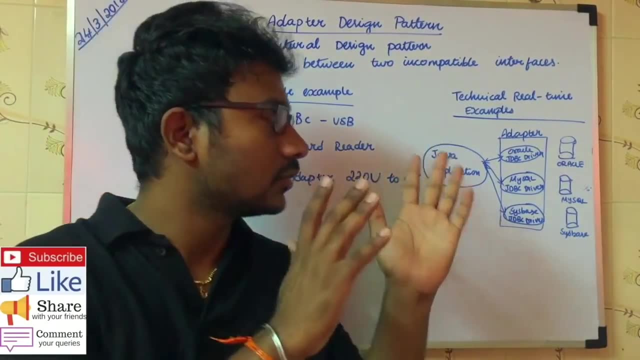 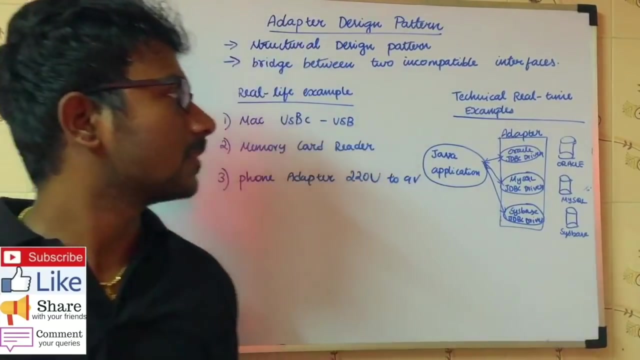 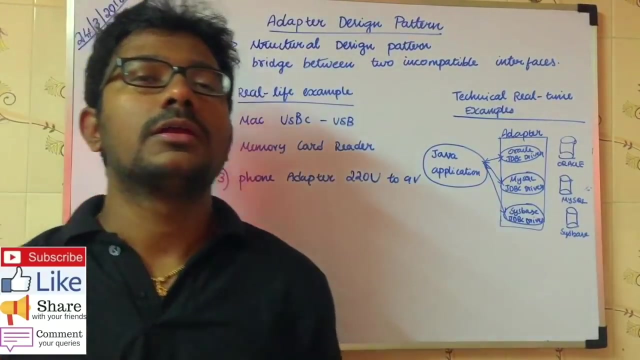 some statements, some mysql, some sql statements, that adapter class would handle those problems. that will handle those things. for example, suppose, if you are trying to migrate from oracle to sysbase means that adapter cache will be changed. so this should be, and by this adapter class. so this is the real time technical example. we'll try to cover the implementation in. 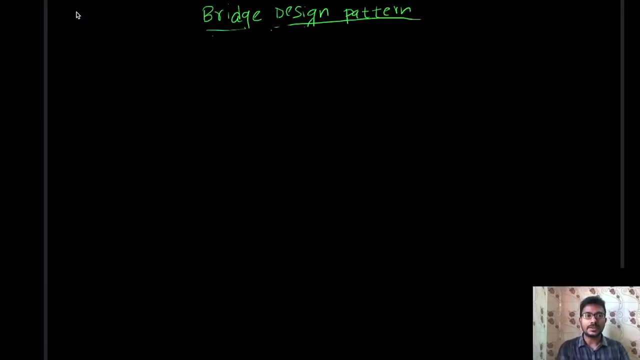 that this is our case. now we are going to see what is bridge design pattern in a detailed manner, using real life example and real-time examples. in the next video we will try to write a java implementation for bridge design pattern. so in this video we will talk about the theoretical content, about 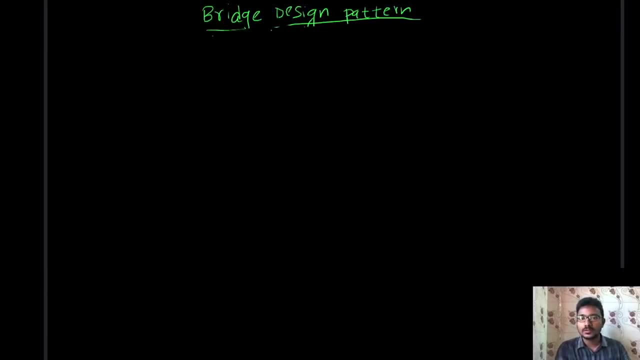 bridge design pattern using some examples. so first, what is a bridge design pattern? before going to discuss about bridge design pattern, we first we will see what is a bridge. generally, the bridge is used to overcome some hurdles without knowing the internal implementation. for example, if suppose you consider this is a leg and this is a bridge, if suppose, if you want to cross this leg, you 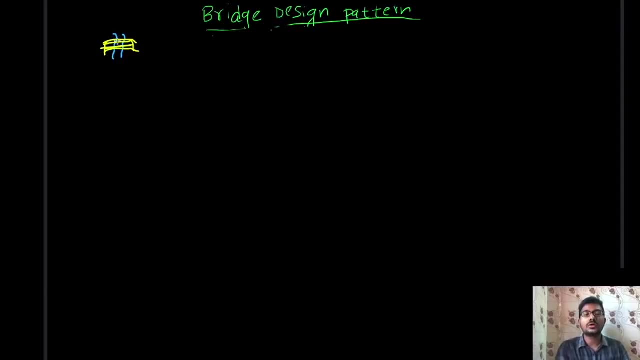 use this bridge and you can cross the bridge. you don't want to know the architecture or the materials, raw materials that are used for constructing this bridge and etc. so you know, you just need the bridge to cross this leg. you don't want the internal architecture and other stuff for 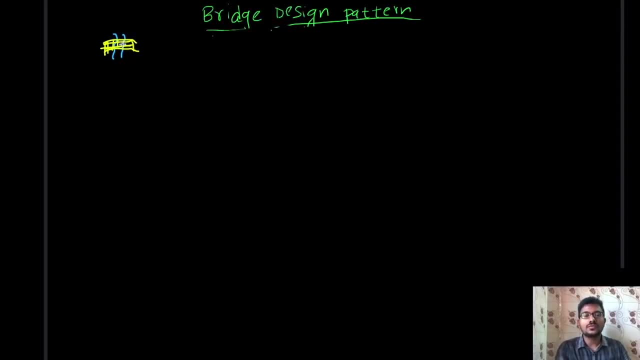 crossing the bridge. so here this is called abstraction, so we are ignoring the internal architecture or inner details about the implementation. so, similarly, if you take any software, there could be two, there would be two layers: one is abstraction and then implementation. so what is abstraction generally? suppose if you 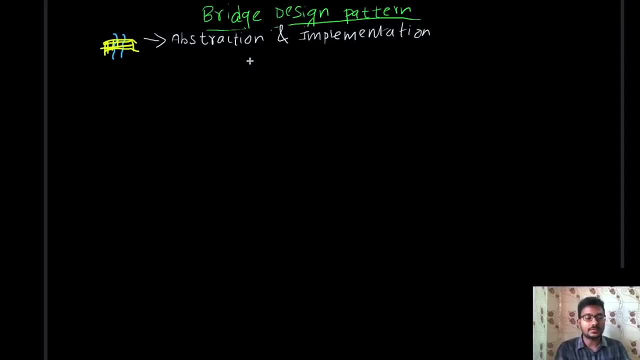 develop any software. if suppose if you are using any aps, for example. if suppose if you are using java eps, for example. consider the map sort, example, if you are using map, or if you are using any of those collections like map release, and then what link release, etc. you don't want to. 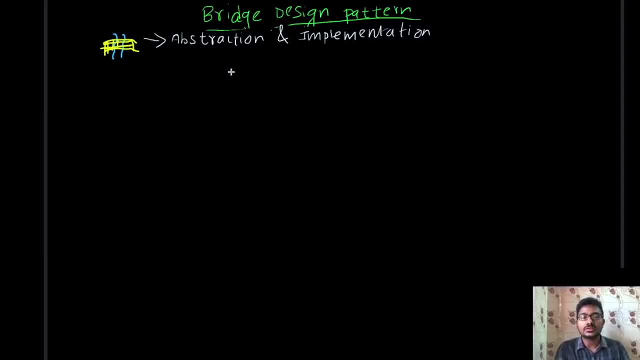 know the inner implementation details about that. you can just recall the methods like dot hat dot, had all dot put, dot put on, etc. so the inner implementations would be taken care by the java community. similarly, here that is called abstraction. you don't want to know about the inner working. 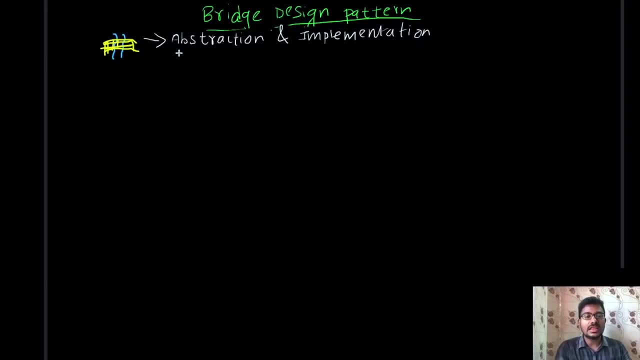 details but you can call them as abstract and you don't want to know about the inner working details for using that, those APS in real life example. we can consider a fan example. if suppose, if you want to run the fan, you can just switch on the fan. you don't want to know the inner technical details. 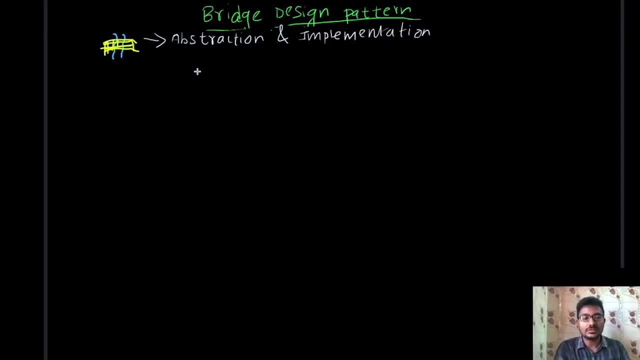 about the fan. for example, what are the raw materials used for, what are the coil which is used in the fan? and then what is motor condition like that? you just want to run the fan. you can just put on the fan. you can just put on this. which of the fan it will run. so here it is called. 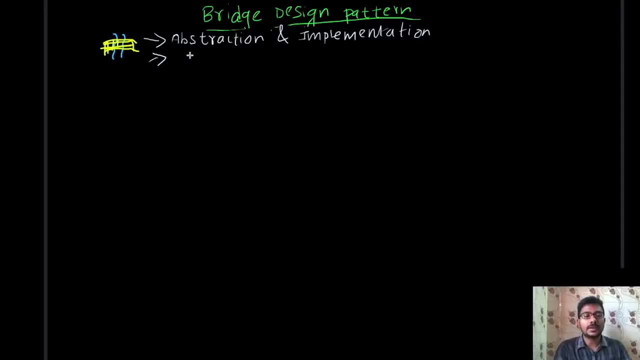 abstraction. so this bridge design pattern comes under structural design pattern. so structural design pattern is one of the important three categories of design patterns. this is called structural design pattern. so here the main concept, a main motto of the bridge design pattern is to allow the abstraction and implementation to happen. 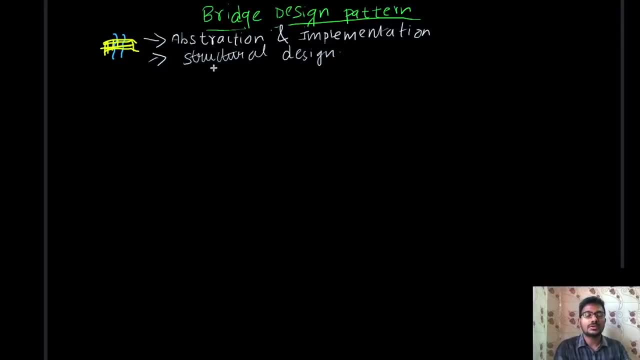 independently. so the abstraction layer can be written independently without knowing the implementation details. similarly, the implementation detail implementation can be written without knowing the abstraction detail, so both can be independent. so for example, let's consider an example. so if suppose if you are a software developer and if you are using some software api's for writing an 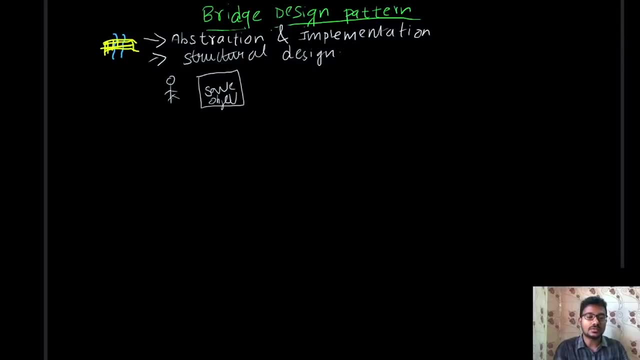 object. for example, you are writing an object, same object. you are just calling the object. you are just calling that method. call save object. this is called API. you are calling this API. so here, this API. initially they have used file to store the data and then, after two years, what they did was they have. 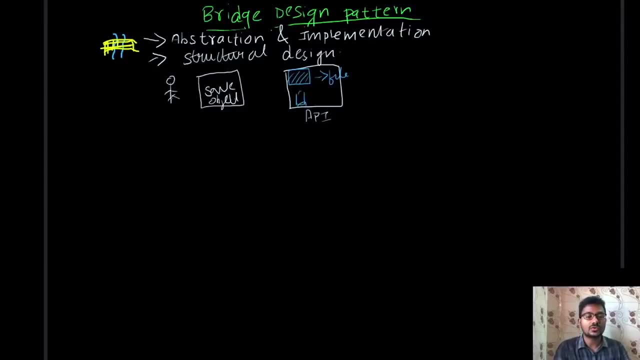 upgraded this file mechanism to database mechanism so they have used MySQL or someumpy sql database for store ár the objects here. these details would be abstracted to the client. so if the client can just call save object, the inner technical details can be handled by those implementing. implementing: classes are implemented. implementing: 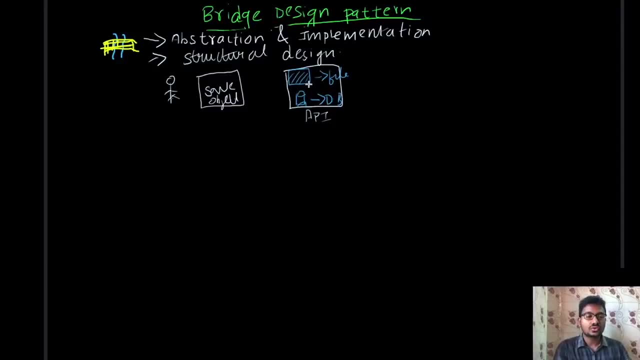 apis here you can throw any implementation at any time without affecting the abstraction layer. so client don't want to worry about those things, it so if suppose, if the after two years, if suppose if a new technology comes, then that implementation can be upgraded to new pigmentation. so here, 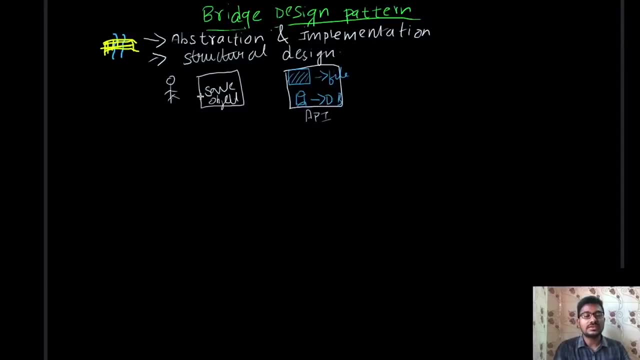 database can be replaced with some other new technology. so here the client need not to be worried about those things. you can just call save object. the inner things can be handled by the those implementing classes, and then it suppose, if the client is called asking about get object, similarly what? 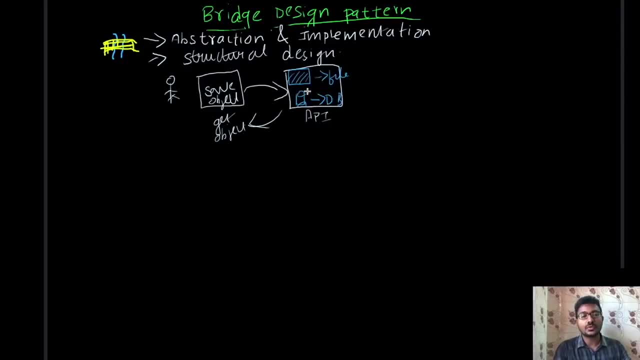 would the you. if suppose that the object was stored in file, then the object would be straight from file. if suppose if the object was stored in database, then from the database that object would be derived. so the client need not to be worried about the inner mechanism. you can just call those API. 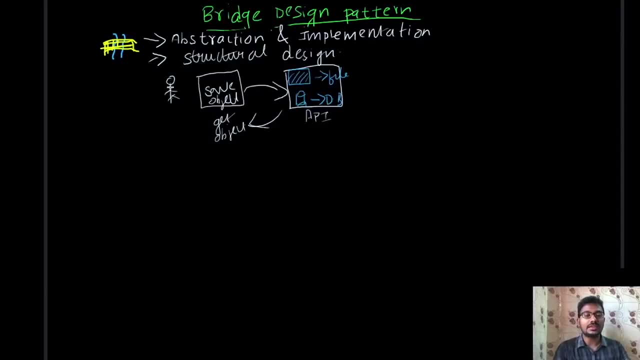 methods. you can just abstract this client as the abstraction over the implementation. this is one of the important examples where bridge descent pattern is playing again Major. and consider another example, built on just another real-life example: it suppose if you are a retail shop owner, suppose what. 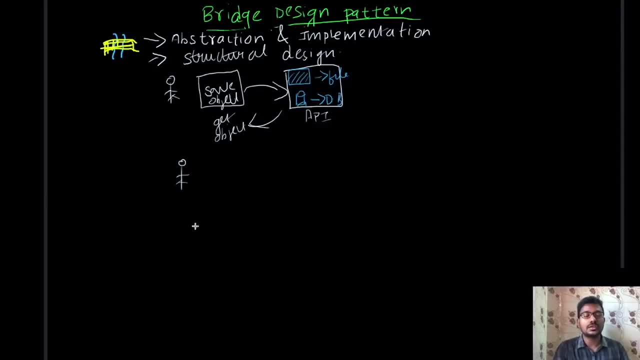 you do is you send message to the customrike, regular customers, regarding the new products which have whenever it comes about retail shop. so you need to automate the customer via SMS or E-mail or Facebook messenger, Twitter. the one way is to add any layer object and you make image data out of thaticy image file. 아니에요 OVERDไป之. 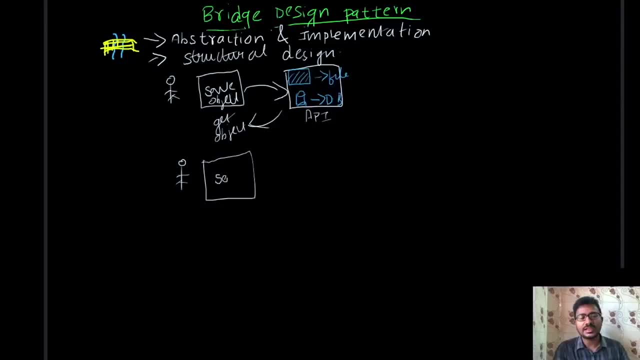 you don't have any technical knowledge regarding that. so what you do is you have bought some software for doing that. you could just click on send message here. the inner technical details are abstracted from the implementation. that would handle all the technical details. for example, if suppose, if the end 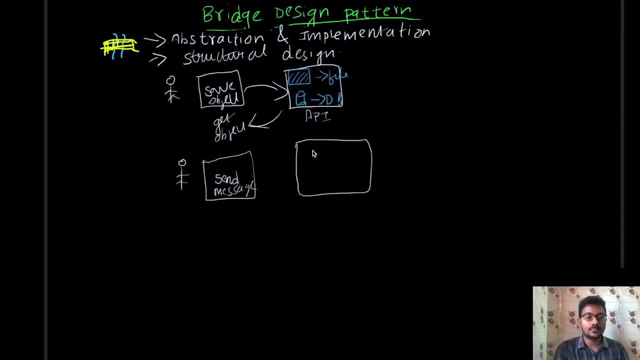 customer uses mobile, then when you click on send message, then the SMS would be sent to the client. if suppose if the end customer uses email means, then this trigger, this triggering button, would send the email to the end client. if suppose if the end customer uses FD means, then we are using messenger. this 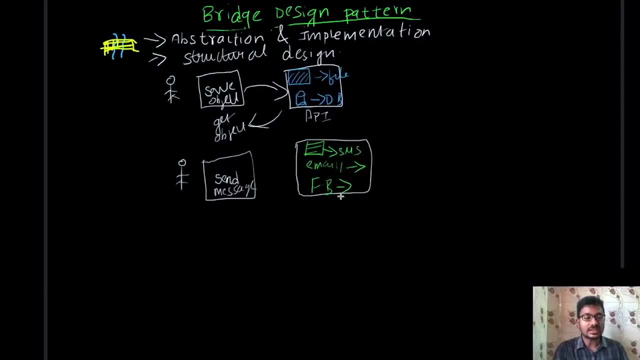 and message would be sent. so here the technical information would be hidden for for the client. so the client can, the client can just call some method to use those technical information. so here the technical details are abstracted for the client. so these are the some real-life examples where bridge design pattern is. 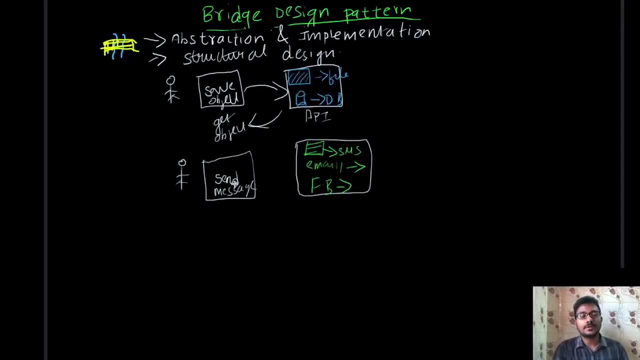 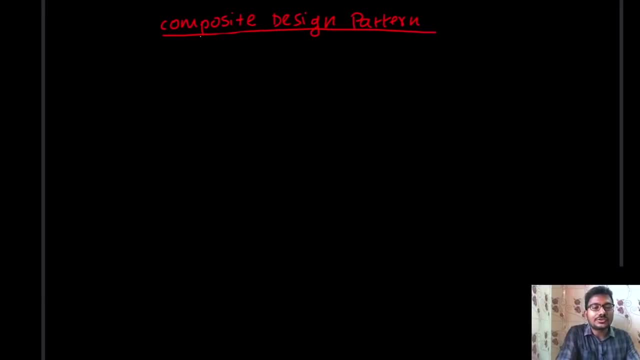 playing a major role. we will try to implement some sample code using bridge design pattern in the next video, so please stay tuned. want to discuss about composite design pattern in the next video, so please stay tuned. want to discuss about composite design pattern- real-life example, real-time examples, definition and then 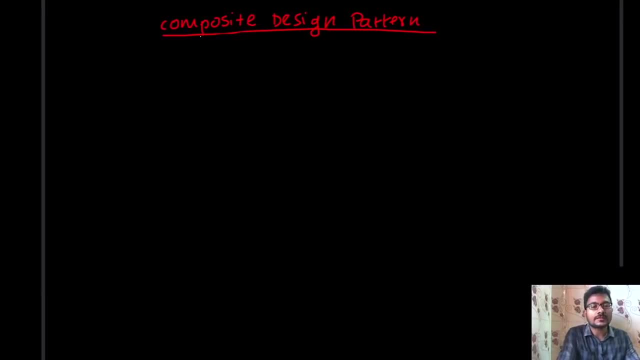 in the next video we will try to this. we will try to implement a sample program using composite design pattern. so for now we will just really we will just try to cover the theoretical information about composite design pattern and using real-life and real-time example. so before that, this composite design 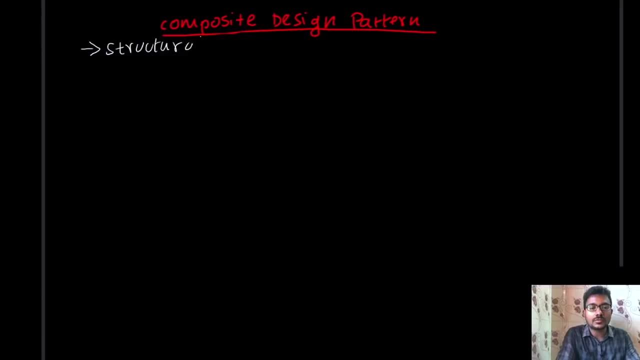 pattern falls under structural design pattern. so, which is the one of the important interview point of questions? so it is which this falls under structural design pattern and then composite design pattern. the main category, the main motto of composite design pattern is: it's up. if our object can be represented in through a structure, then it can be considered as 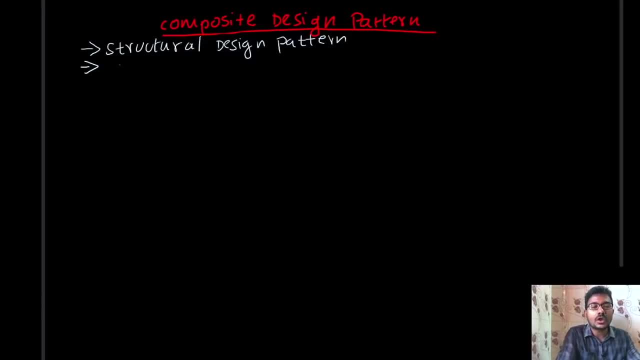 composite design pattern, so you need to represent the object in three structure. object in three structure, so it, for example, we can consider some diagram like this: so this is your object, this is your complex object. if your preset can be represented in three structure, then you can consider as a 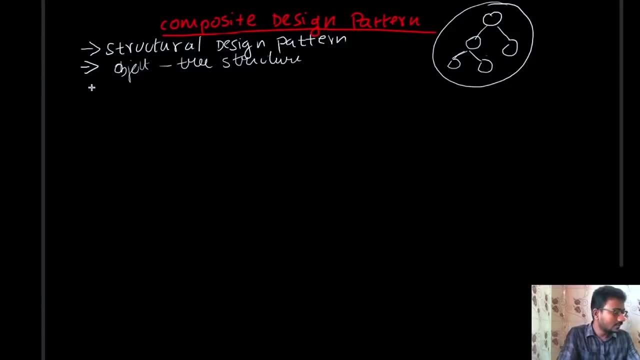 composite design pattern. and then the second rule is the nodes are classified. and the second principal is that nodes are classified into two types. one is composite and then another categories live. so this is called composite design and this is called lift. we will try to explain those things using some real life example. if 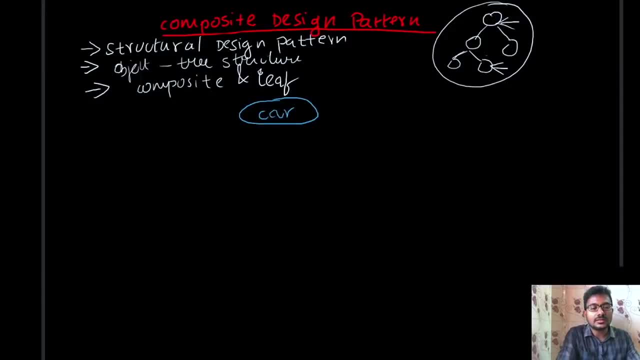 suppose, if you are buying any car, then the car would have engine, and then the car would have tire and for that engine, the it could, it would have made up of some electrical components, and then that engine would have some valves and then that electrical components would have. 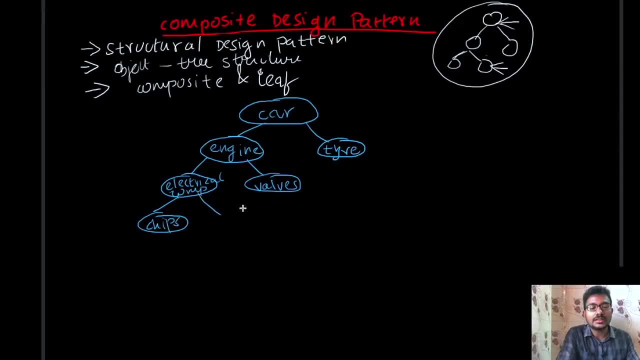 some electrical chips, and then that electrical component would have some transistor transistors and then this is some tree structure of some complex object called car here. if suppose, if some operation can be applied on a leaf object, then that operation should be applied on a other composite and other leaf objects also. so first, before going to that, first we'll try to. 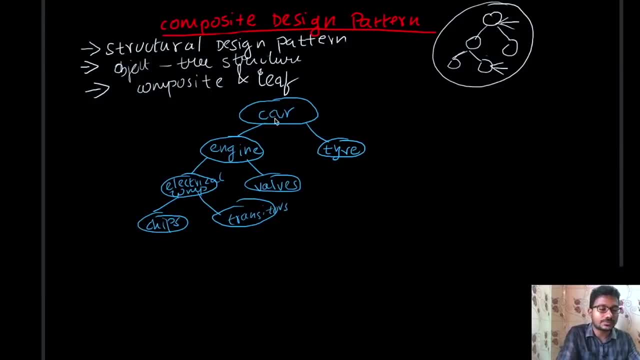 classify the composite and leaf objects in this complex object. a composite object would be car engine, tire. sorry, car engine electrical components are the composite object. the reason behind that is: a composite object is object which contains which which would be having some child objects here car is having engine and tire as a child, child objects, and then engine is connected, is having electrical. 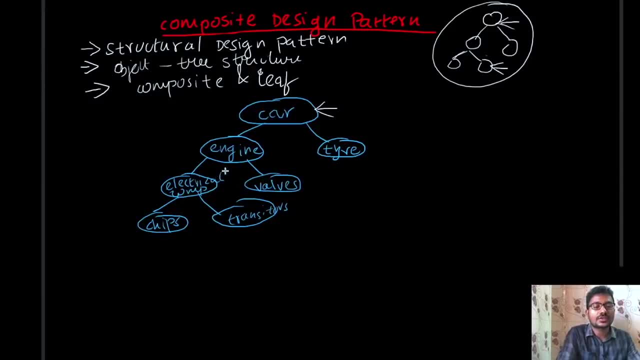 component and valves as child objects, whereas tire valves, transistor chips are not having any child object, so these would be considered as the leaf objects. so any object which is containing some child objects would be considered as composite object and objects which don't have any child object would be considered as leaf objects. so here tire valves. 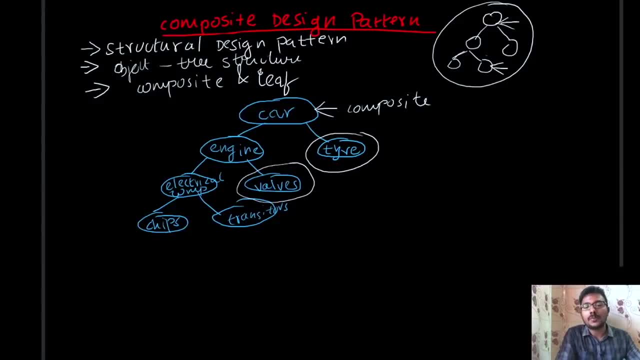 transistor chips are the leaf object. if suppose, if you apply, perform some operation on the child objects, for example, get price is the operation which is a method which can be applied on transistor object, chips, objects, valves, tires- here this create the price operation are being applied on all the leaf objects, then that operation should also apply on the composite. 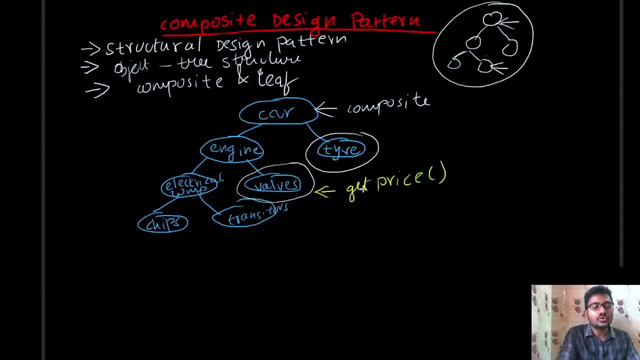 objects called car, engine and electrical component. so you can get the price of transistor, get the price of the chips, you get the price of valves, get the price of the tires, engines, electrical components, cars and etc. so here the operation which is applying on leaf object is also applying on the 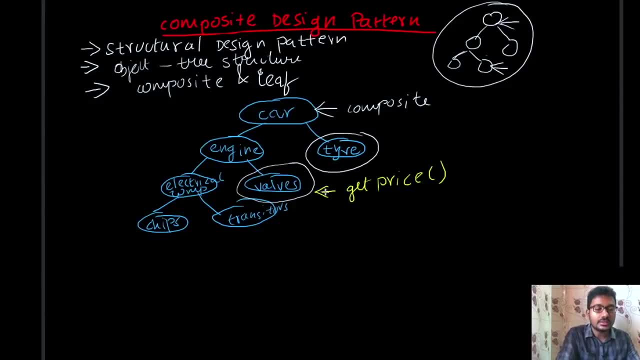 composite object and other leafs and other composite object, then this would be considered as a composite design pattern. so these are the two principles and rules that are needed for qualifying the so for an object into composite design pattern. there are various criteria, there are various use cases where 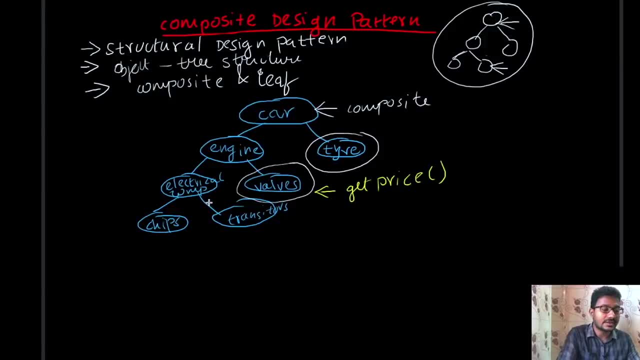 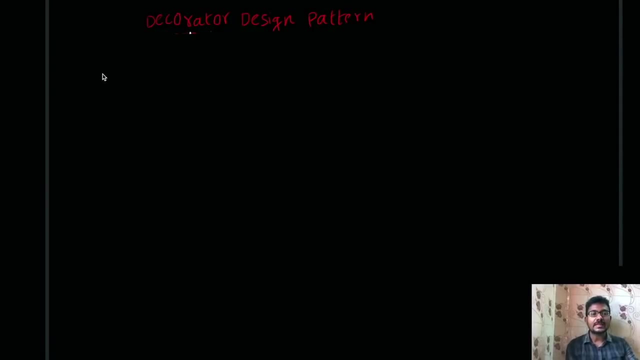 we are using where we would use composite design pattern in real life examples to solve real life problems. we will try to cover one of those real life problems using our implementation in the upcoming videos, so please stay tuned to this channel. now we are going to discuss about the decorated design pattern in a theoretical manner using real life example. 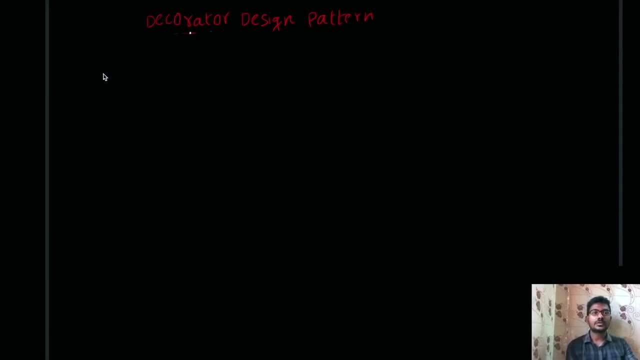 and real time example. in the next video we will try to cover the sample program to explain decorator design pattern in a detailed manner. so first, what is a decorator design pattern? so this decorator design pattern falls under structural design pattern, so structural design pattern. and then this decorator design pattern is used whenever an object behaves, whenever an object 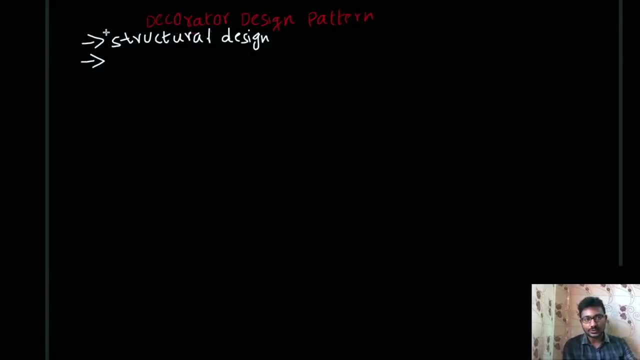 needs to behave dynamically at runtime based on the structure of the object, using decorator design pattern on the request. then we can use take a decision pattern. so, for example, this is a definition: additional responsibilities for an object at runtime. so we are adding additional responsibility for an object at the runtime without affecting the base object. that's important- without affecting the 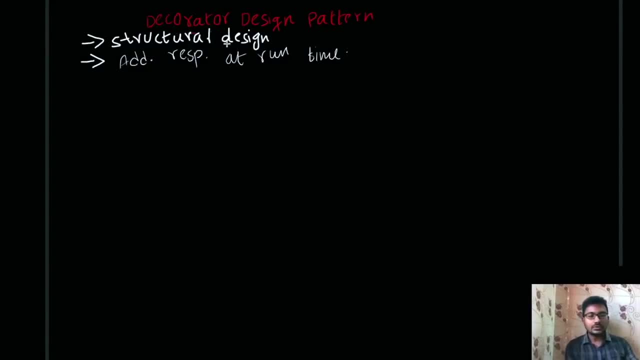 base objects. that's the important point. so we will try to explain about this using some real life example. so, for example, if you are going to some supermarket and if you are buying some cone, what you do is you would ask the customer, you will ask the food server to serve the ice cream based. 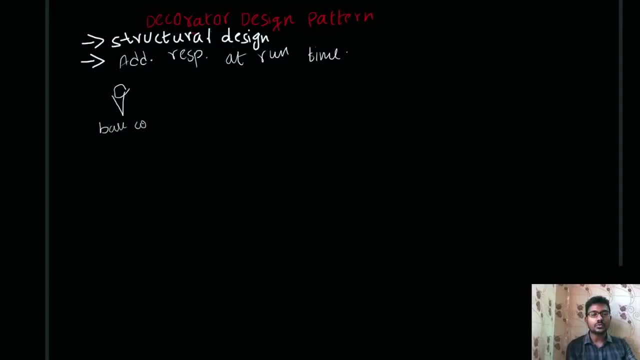 on your request. so this is base ice cream or base cone. if suppose, if one of the customers asking the i need some vanilla ice cream, so what that food vendor would do is he will try to use that base and then, if you, you will try to fill the vanilla ice cream. so here there is a base object. this base object is: 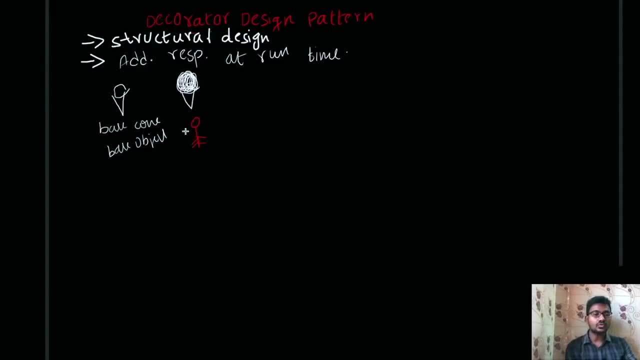 converted to custom object based on user request. so here the base object is added with some additional responsibilities. here vanilla ice cream is the additional responsibility at the runtime. so this is one of those example. suppose another customer is coming, another customer is asking about. he is asking that he need, he needs him. 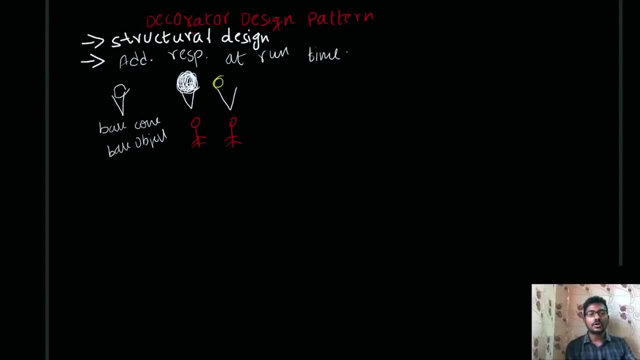 chocolate ice cream. so here the vendor is filling the chocolate at the runtime. here chocolate is the additional responsibility added to the base of the at the runtime. so this is the another scenario in our real life. so we will try to cover another example. if suppose this is the 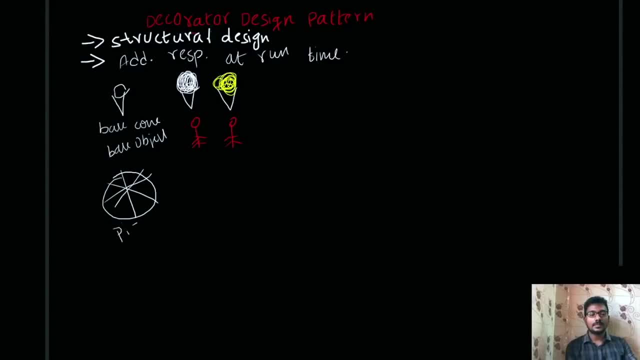 plain pizza and if a customer is coming to the pizza shop and their customer is ordering, i need here the chef food chef. what you do is he would take the base object, which is a plain pizza, and he will add some extra responsibilities- in our case, which is chicken at the runtime- dynamically. 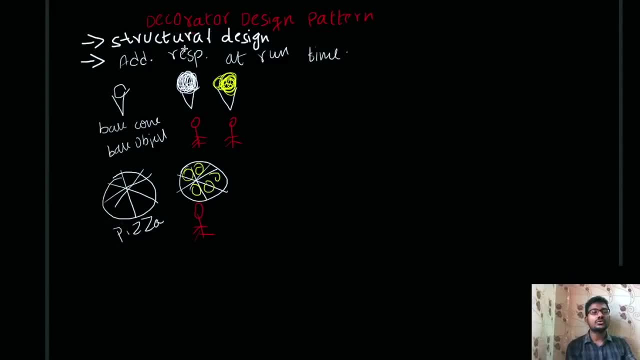 that's important. that's the more important when comes to decorated design pattern. so decorated design pattern should be used, a decorated design pattern. so whenever an object should be treated dynamically at the runtime, based on some criteria, then we can choose the decorated design pattern. so we will try to cover decorated design pattern java. 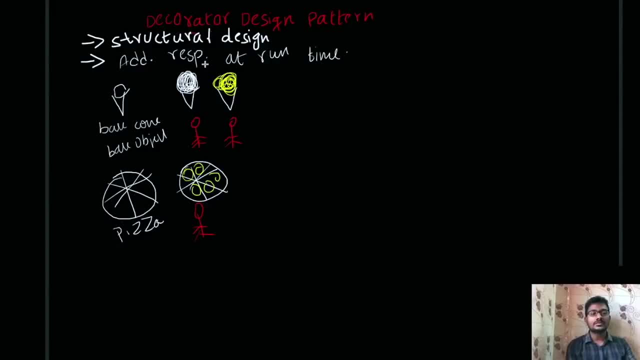 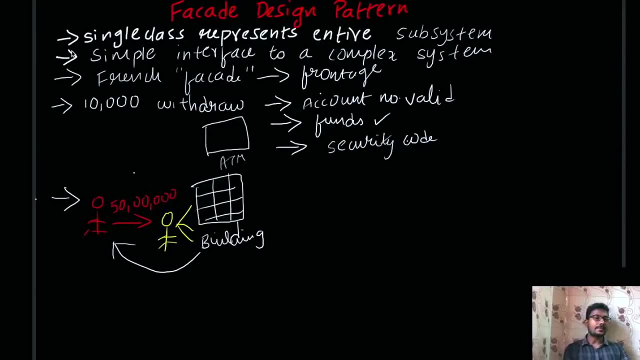 implementation in the next video. please try to watch that video also for better understanding. so thanks for watching this video about facade design pattern in theoretical manner using real life and real-time example. in the next video we will try to write a sample program to implement the facade design pattern. so first, what is a facade? in french facade meaning is frontage. so 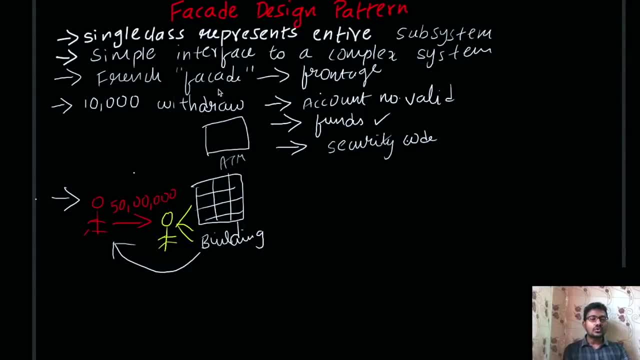 whatever you see is called facade. so the main mode of behind the facade in the design pattern is simple interface. simple interface to a complex system. so the system can be complex, but you need a simple interface to operate the operations. so another principle is single class represents entire subsystem. so your system can be, your system can contain n number of subsystems, but 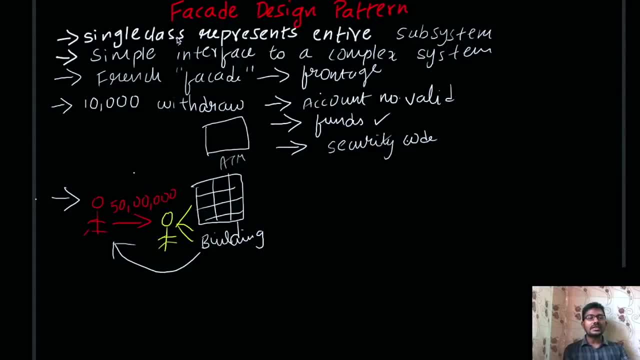 the end user should see as a single thing. entire complexity should be handled by the inner implementation. you don't need to worry about that. so this is the main motto beginning the first high design pattern. we can explain that using some real life examples. the first real life. 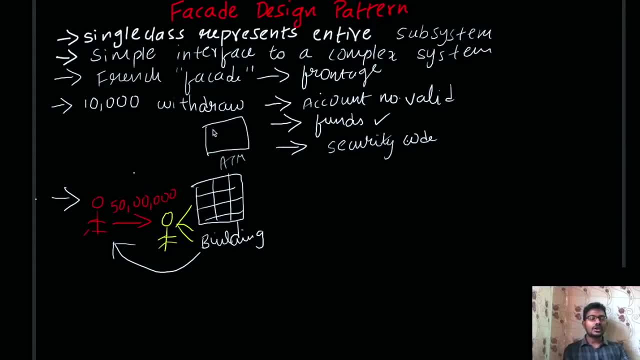 example is: if suppose if you are using ATM, if you are trying to withdraw some amount from ATM, for example 10,000 rupees, so what you do is you would, you would insert your ATM, you would insert your bank debit card into the ATM and you would give the required pass, required password, which means passcode. 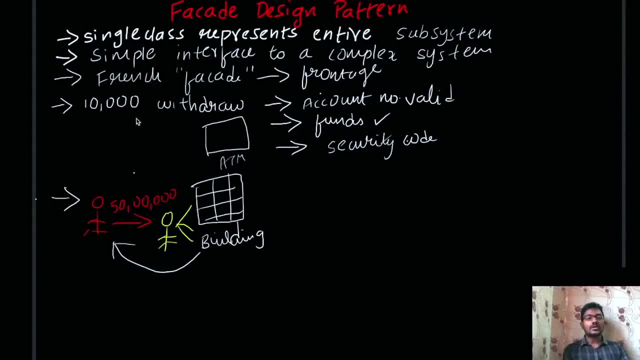 so here, once you do that, once you trigger 10,000 rupees withdraw button, then these are the following things that would happen behind this scheme. so first it will check whether the account is valid or not, and then it will check whether you, your account, has some of sufficient funds for withdrawing 10,000. 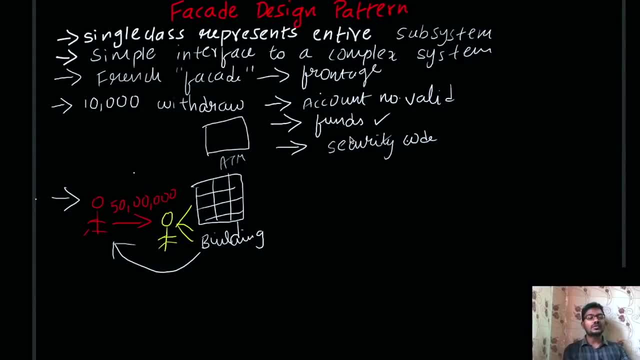 rupees and then it will check whether your account, your PIN code, is correct or not. so after validating all these things, then 10,000 rupees would be withdrawn from ATM. so these are the complex things that handle behind this scheme. for the user, for the end user, this interface is very simple. you can just click on some button. 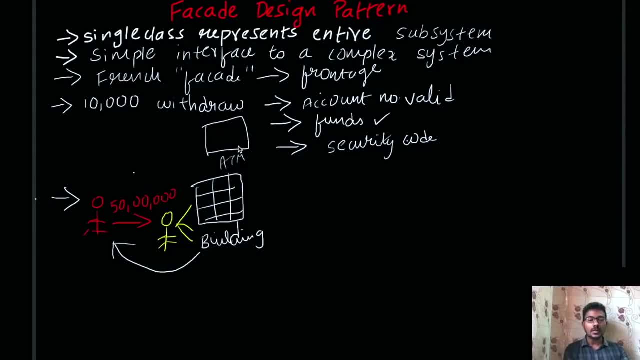 and you can just give the amount of amount that you need to withdraw the interface very simple. so this falls in the first high design pattern. so simple interface to a complex system. so another example: if suppose, if you are trying to build a building, so for example, that building consists of ten floors and each floor 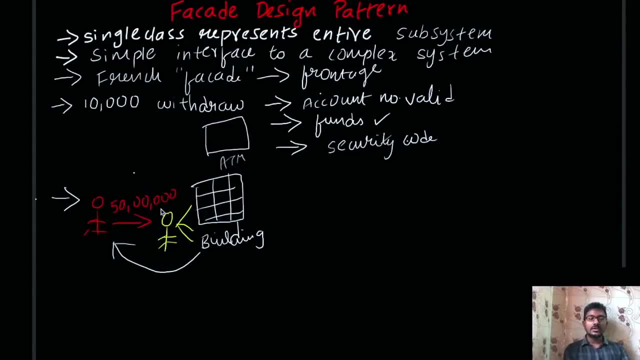 should contain some two or three rooms like that, and then, for the quality purpose, you would need to select the better bricks, cement and etc. here you would, too, call to build this building. you need to maintain many things, and that's a very complex process. so what you are trying to do is you are trying. 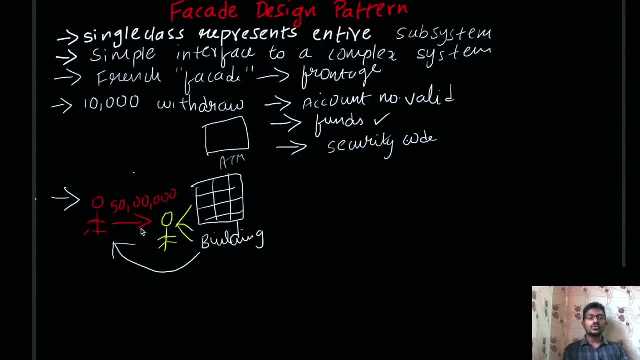 to give this contact to the building contractor. so who would manage that these things in a better manner? so what you do is you are trying to give 50 lakh rupees to the base building contractor and you are explaining well use cases through this building contractor. 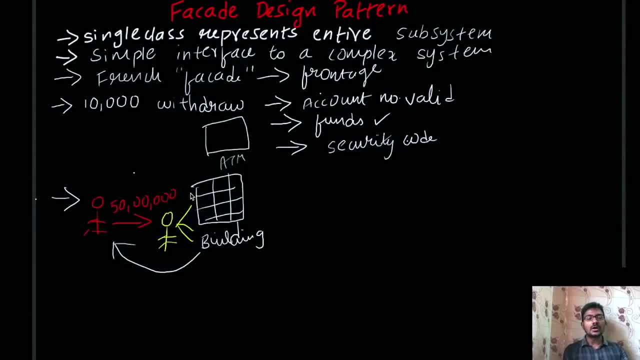 then this building contractor would handle this. complex things behind the scheme. the end user don't need to worry about this. that's building contractor with worry and manage these things. so here this is another real life example where facade design patterns is applied. so here this is the end user. you need not worry about the complex things behind the scheme for building. 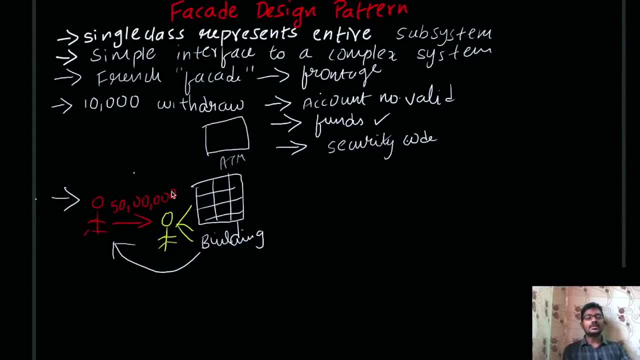 this building, the everything would be managed by this building contractor. so this is another example where facade design pattern is applied. so in the next video we will try to explain facade design pattern using some sample implementation using java. so thanks for watching this video. now we are going to discuss about flyweight design pattern: theory principles and real life examples. 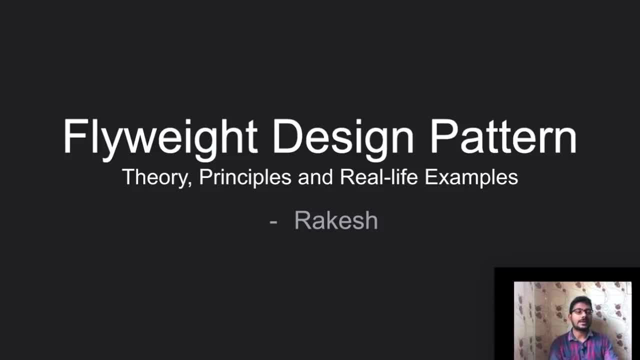 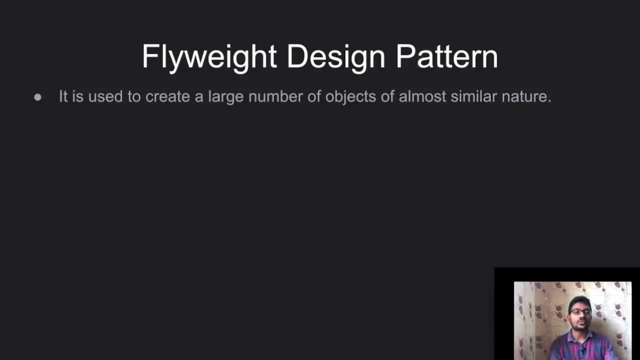 in the next video we will try to cover the flyweight design pattern practical implementation using java. so first, the definition for flyweight design pattern is: it is used to create a large number of objects of almost similar nature, for example, if suppose, if you are going to, if you, if you need some thousand. 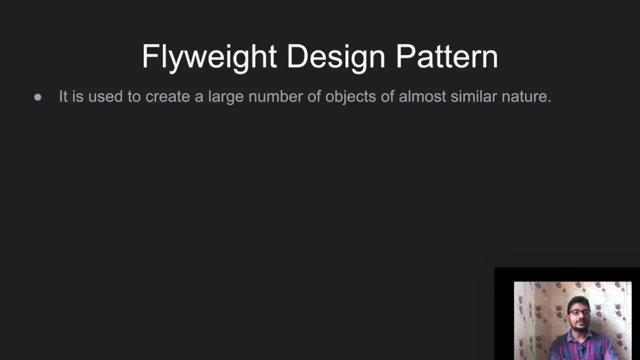 thousand copies of some data. the data is in our system. so what we will do is there are two options. so first option is: we will try to get the printouts for thousand times so we will get the expected output, which means thousand copies of actual data. the 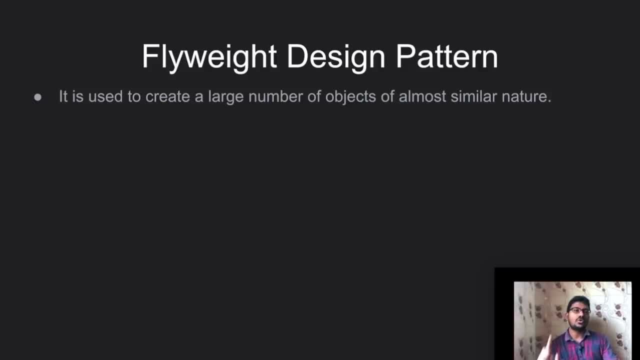 other way is we can get printout of one copy and then we can use that copy for uh, for taking the jar's copies or for other remaining 999 copies. so by doing the second way we can share some amount of money. money, for example, if suppose, if the shopkeeper is trying to uh demand one or two. 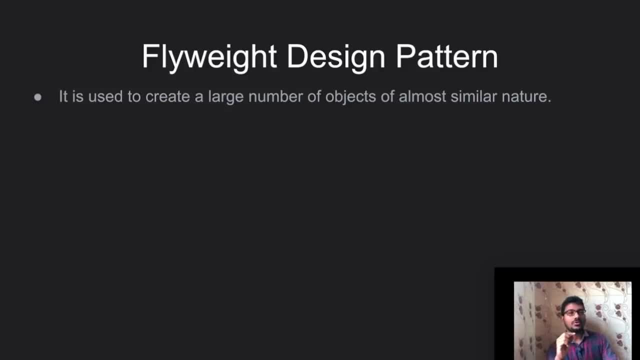 rupees for a print, uh, for a copy for printout, then thousand into two rupees, then the total amount, that total amount that we need to pay to the shop owner, is two thousand rupees. if suppose, if we take one printout and then if we, uh, if you do, if you ask the software shopkeeper to do the 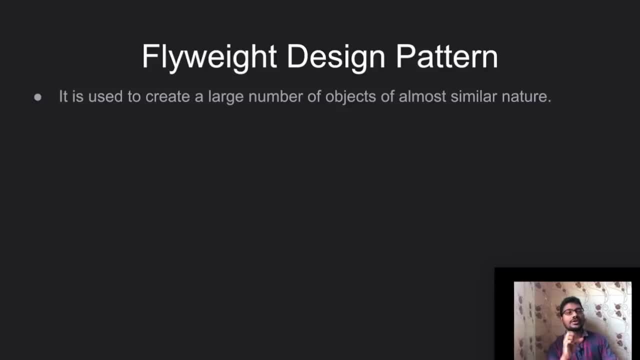 jar's copies of the for remaining amount, remaining quantity, which means 9999, then we could save nearly thousand five hundred rupees. so in this way we can save nearly thousand five hundred rupees. so in software angle, in software applications also, we can reuse the something. if we can reuse something. then we can save memory. so by saving memory it eventually saves the. it improves the performance. so five way design pattern is one of those which saves some amount of memory by reusing the existing objects. so it is used to create large number of objects of almost similar nature. 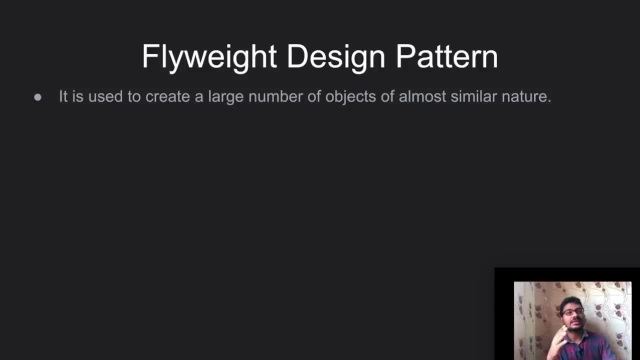 if the objects are in similar nature, then we can create n number of objects without expanding the memory, without bombarding the memory. we can reuse the objects. the second definition is: large number of objects consists large amount of memory. the second point is: so there is no large amount. a large number of objects request larger. if suppose, if one object requests 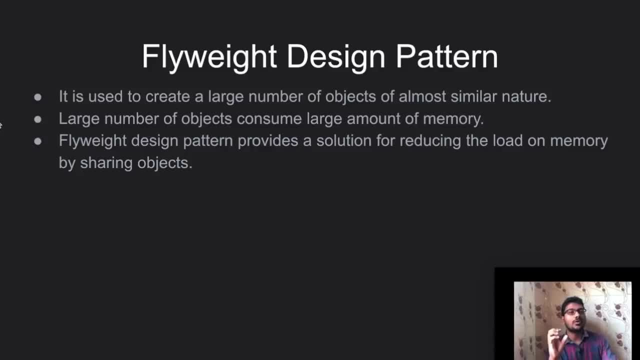 one mb. if, if we equate thousand objects of the similar kind, then thousand into one, we need 1000 mb memory. flywheel design pattern provides a solution for reducing the load on memory by sharing objects. the main thing is to reduce the load on memory by sharing objects. the main 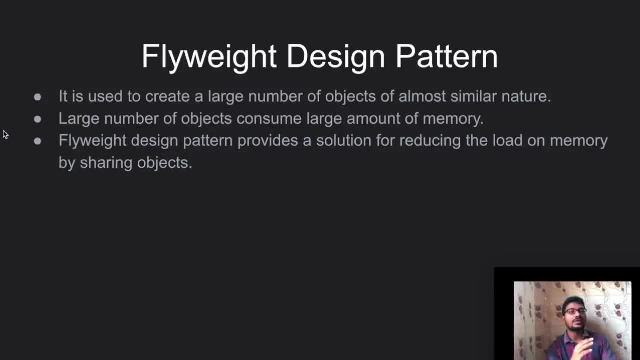 principle began for private design partners: share the object which can be shared. it is used to reduce the number of object created and improve performance. so, whenever, when, if you reduce the number of objects create that are created are getting greater, then we can eventually improve the performance that is directly proportional. reduce the number of objects that improve the performance. 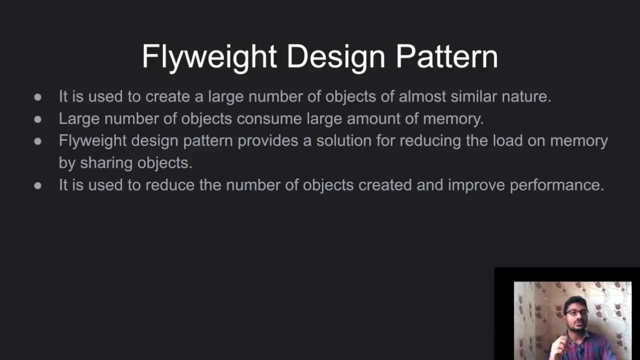 so if you want the better performance, then you need to reduce the number of objects. and the third and the fourth point is sorry if the point is it reuses the already existing similar kind of objects and create new object when no object is found. so we can. 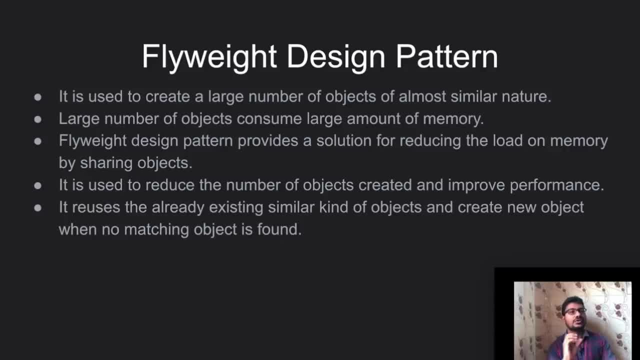 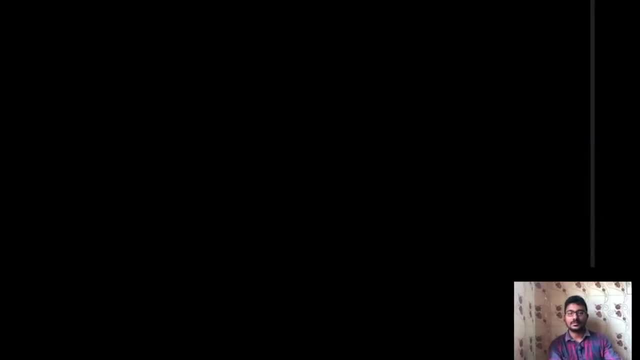 relate this point with the real-life examples using angry birds, so that you could get the information and better manner. so, for example, we would have played angry bird game in at many times. so if I really consider this one one of the angry bird, this is the base angry bird which contains, which has two eyes. 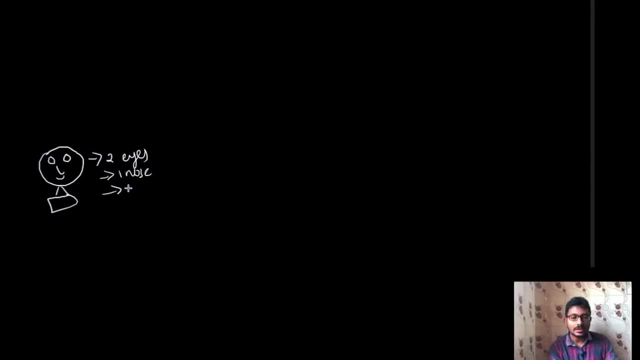 one nose and two legs. these are the features of this angry bird. if suppose if we can reuse this object. if suppose if we need thousands of a similar object, then we can reuse this object. if we require a similar kind of object, for example, we need this object. but 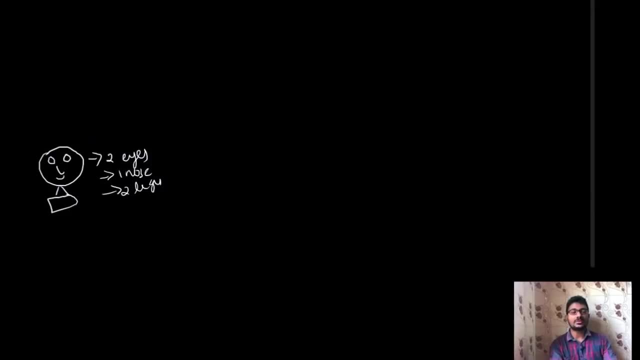 of a red color, then what we can do is we can use. we can use this object from the cache and then we can apply the red color on the flight. so this is the power of flyway design pattern. so we can create n number of objects of this similar kind without expanding the memory. 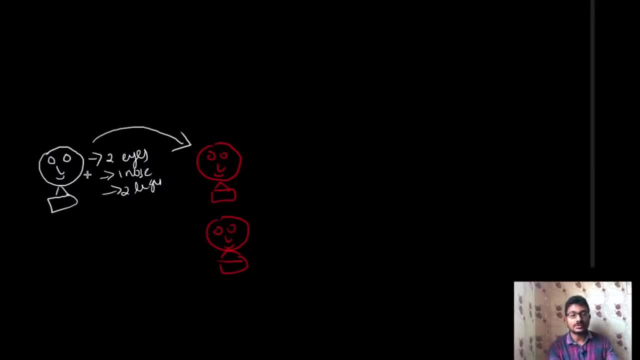 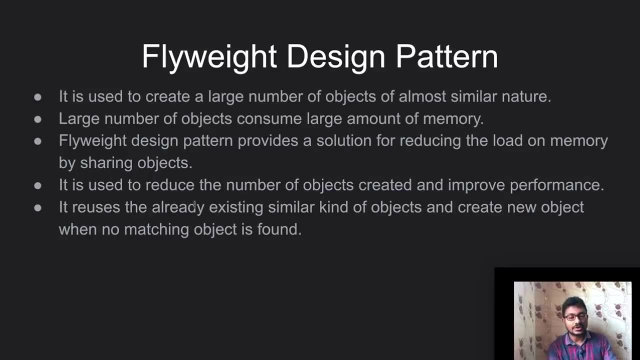 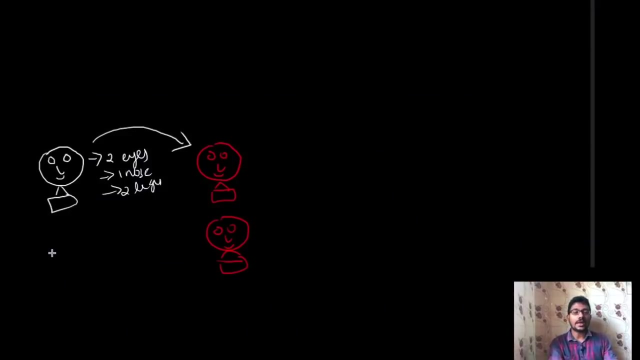 at the runtime. so here we are reusing the object, but we are applying the additional features on the flight. so that's the point: it reuses the already existing similar kind of objects and create new object when no object is found. if suppose if a new angry bird of different dimensions is required at 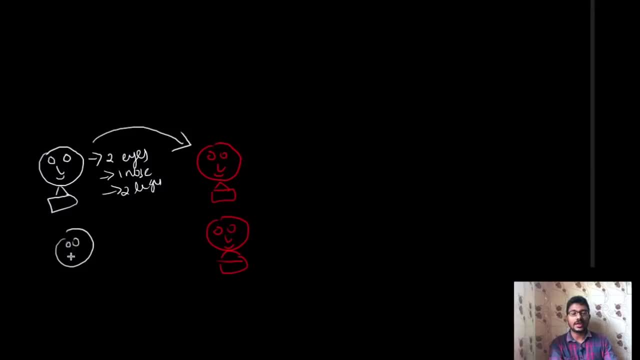 the runtime, for example, if a new angry bird with two eyes, one nose and one leg, two eyes, one nose and two, one leg. this is the requirement at the runtime. we don't have any, any objects of this kind. so what, uh, this pattern says is try to create a new object if the, if it doesn't exist. 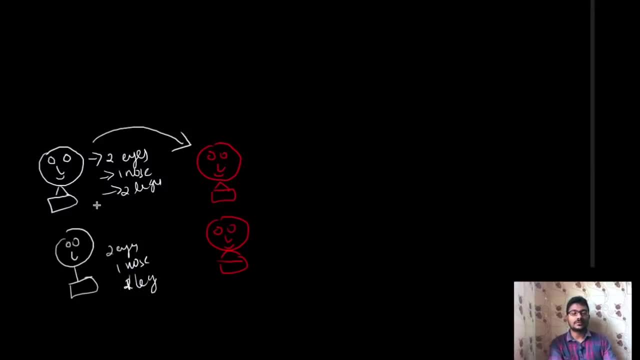 at the cache. so what it will do is it will try to check whether this object is already present or not. if it's present, it will try to reuse that object. if it doesn't present, it will try to create the new object at the runtime and it will try to reuse for the next success you request. so there. 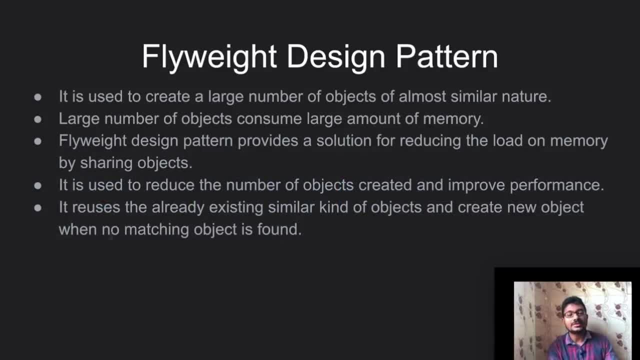 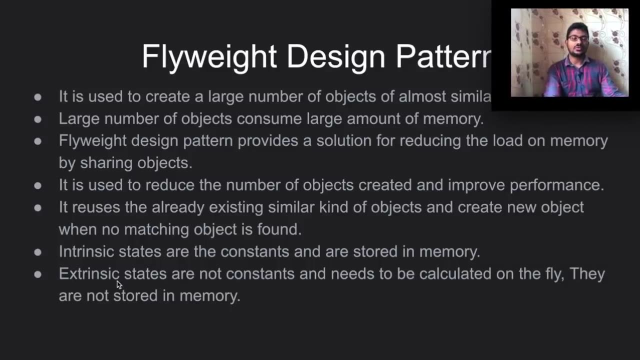 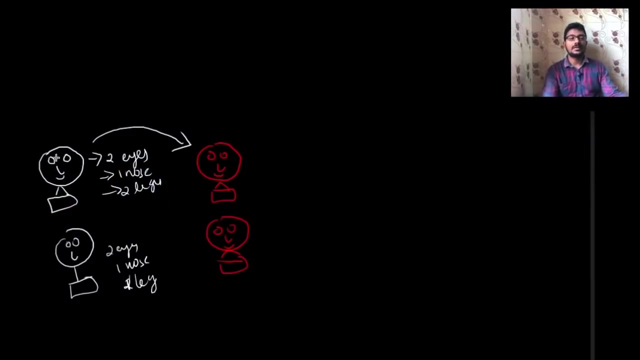 already existing similar kind of objects and create new object when no object matches form and the intrinsic states are constants and stored on memory and extrinsic states are not constants and needs to be calculated and that are not stored in, they are not stored in memory. so here intrinsic states are those there are things which can be saved in memory, for example, 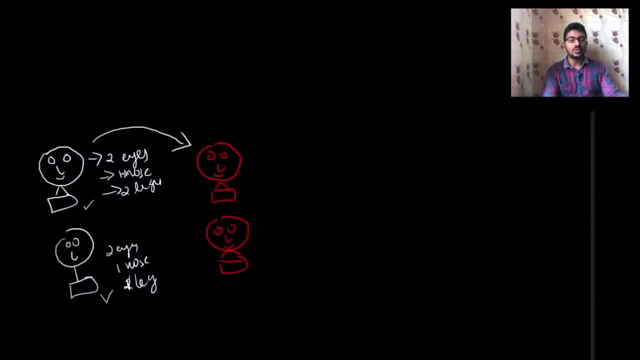 this is one angry bird object and this is another angry, but i've said here two eyes, one nose, two legs, constants that can be saved in memory. here, two eyes, one nose, one leg are constants that can be stored in memory at the runtime. if suppose, if we need two eyes, one nose, two legs. angry bird with. 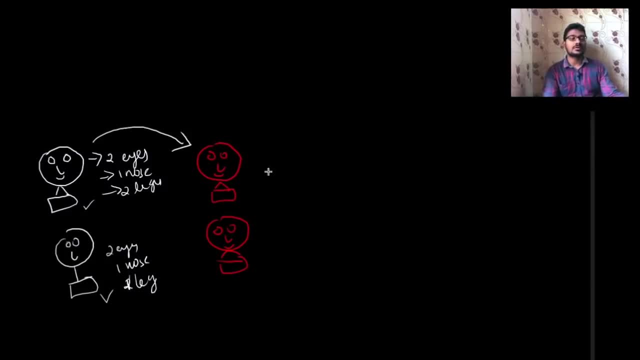 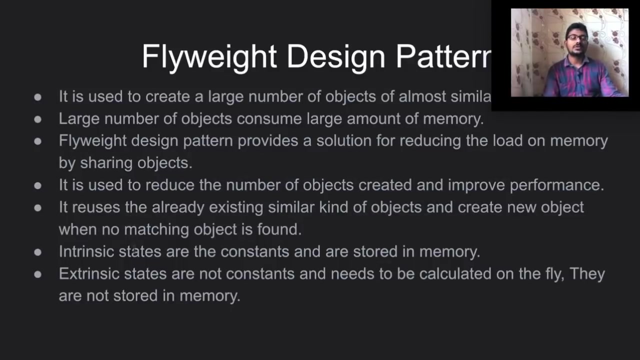 red color here red color is extrinsic states. if suppose, if we need two eyes, one nose, two legs angry, but with the blue color? here blue color is extrinsic state that can't be stored in memory because that i had at the runtime that would be used for that request only, so that need not be. 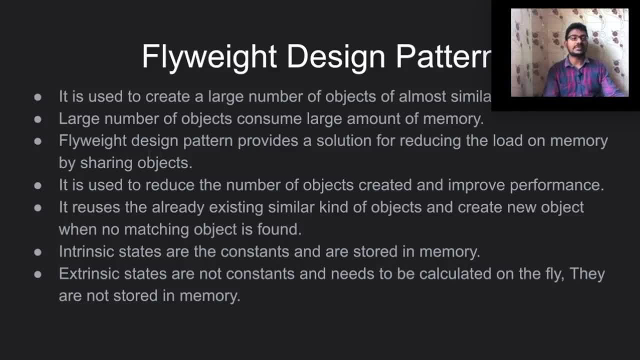 stored in memory. these are the some points about the flyway design pattern. we will try to write a java program for this in the upcoming video. so please stay tuned to this video, if suppose. if you want to learn software design patterns in a detailed manner, then you can download the book. that book link would be present at the description box of this. 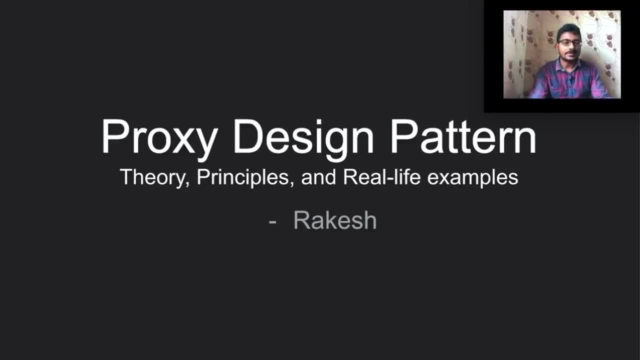 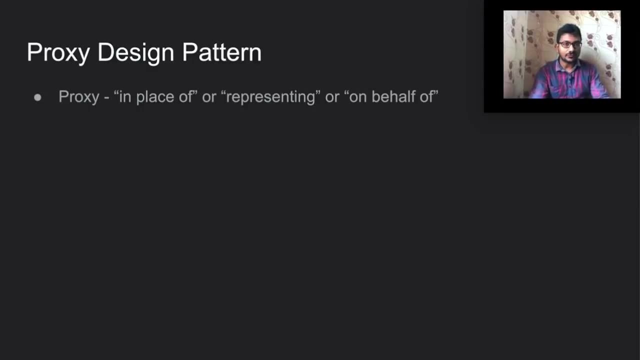 video see about the proxy design pattern: theory, principles and real life examples. in the next video we will try to cover the proxy design pattern and the practical implementation using java. so first, what is a proxy? proxy means in place of, or representing, or or bigger for, so this is the general meaning of proxy, so please try to watch. 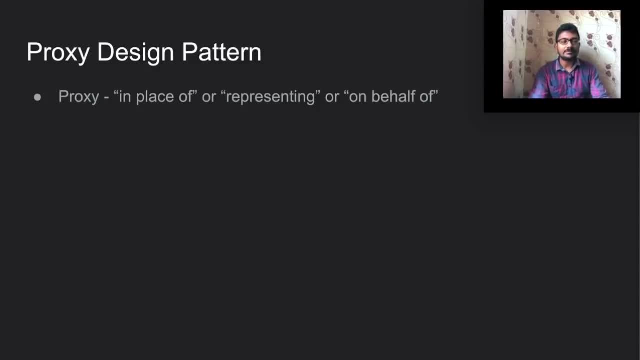 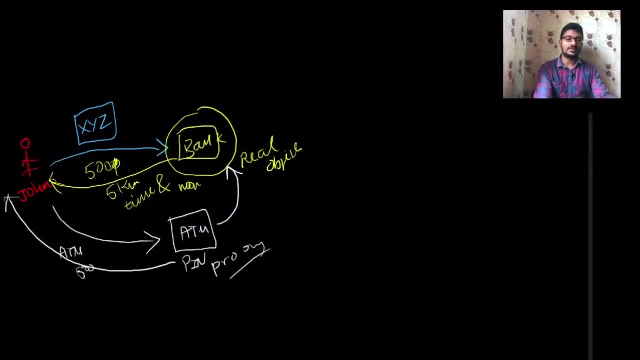 this video completely so that you could get the proxy design pattern in a detailed manner, because i have included the real life example of proxy design pattern, so this is the real life example. this is the illustration of the real life example of proxy design pattern, so please try to. 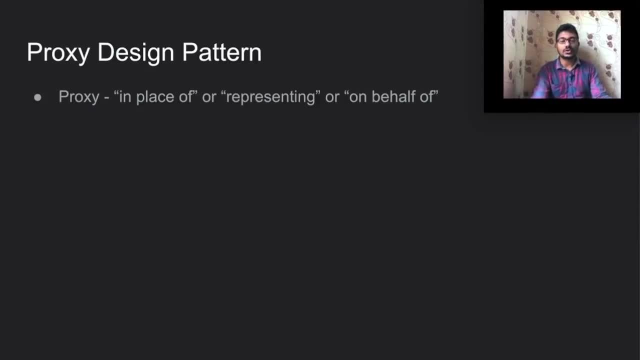 watch the video completely before getting the real life example of proxy design pattern. it does not reduce you to seeing the video completely, java. so that is the real life example. nuana is showing the real life example, java. okay, this one. what is the real life example of? this is the reality, so usually we would. 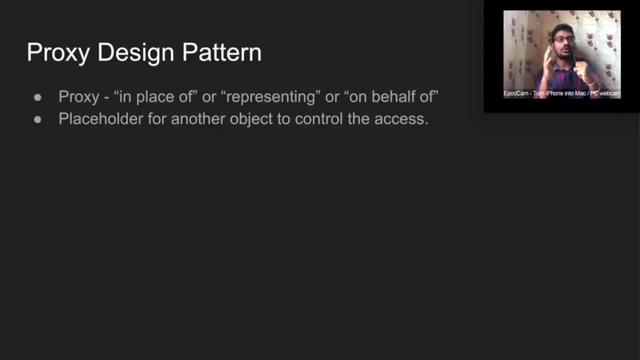 compare a real life example with number. obviously- and we do not use questo as in java, but as is known to, people can use centimeters to last used to. the reason is not counted before object. this proxy object will comes into act and it will try to check whether client has. 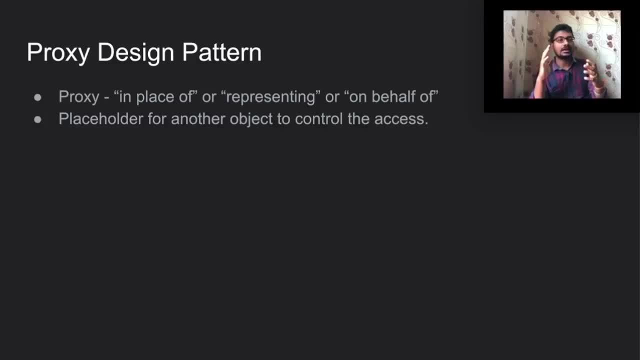 a permission and client can and and other various based on various criteria. this proxy or object will try to reply to the client, whether that client has the access to this real object or not. and then the threat. so proxy is the object that is being called by client to access the real object. 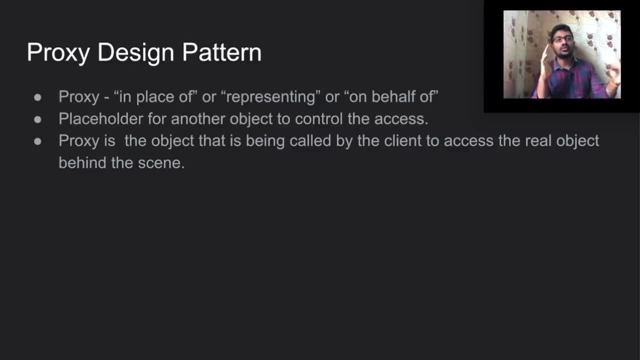 behind the screen. so there is a client. this client knows only this proxy object. the client doesn't aware about this real object. this proxy object will try to manage those, the internal things, and it will try. this proxy object will try to contact this real object and it will try to get the 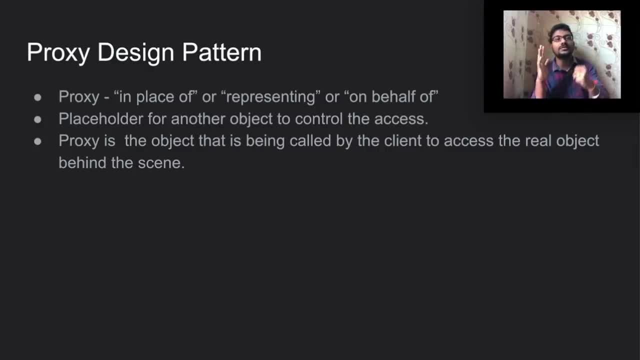 relevant information and data and this proxy will will be showed to the client. so this is second, uh, this is third point, and then proxy pattern represents the functionality of another class. so this is the real object. uh, real object, real class object: the functionalities of this class object, this 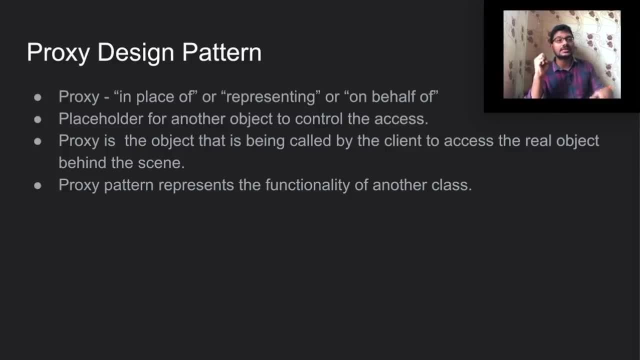 main this. the functionalities of the main object is replicated by this proxy object- virtual. there are three types of proxies that are widely used in industry. the first one is virtual. proxy is a placeholder for expensive to create object, for example, and then the real object is only creative and a client requires. 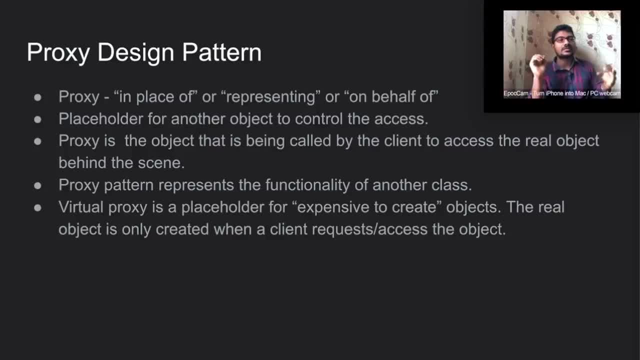 that the client requires themselves to create a real object. for example, if a client is trying to access the student data of a particular student, for example, the client is accessing the student id, one data. here the student doesn't aware about the real object at all. it will write: it will see that. 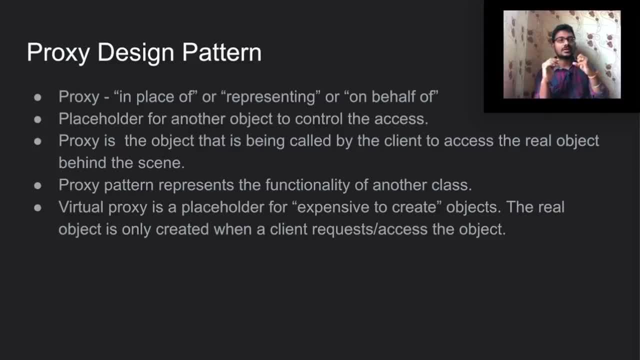 there is some object. this is a proxy of the. the client knows that there are some object that will be served for the request. the client will know the the real object won't be created until the client request the actual thing. actually, until the client request. till that time this proxy would be shown. 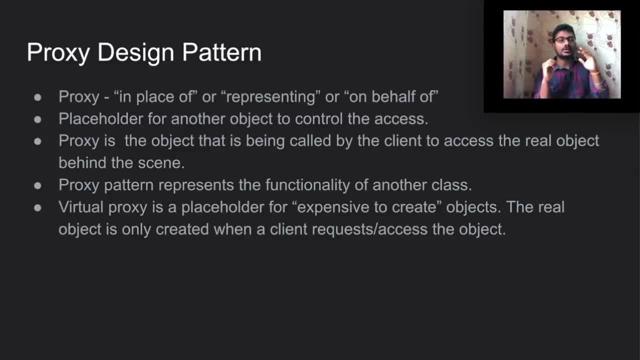 to the client when a client actually requested, when the client actually requires, then only the real object would be created. for example, student id1 is the actual request. during the runtime on the fly, the student id1 data would be featured from database and that actual data would be. 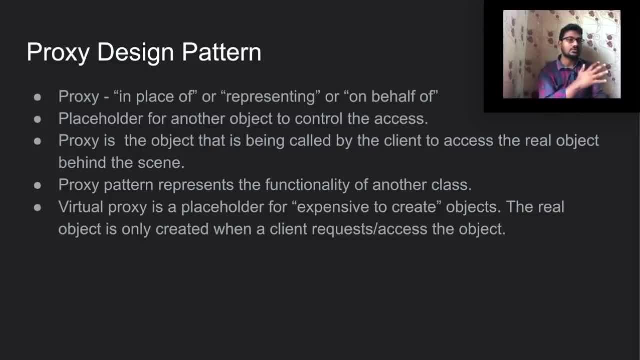 converted to the real object, that real object would be served to the client. so this is the procedure for the proxy design pattern, virtual proxy and the remote proxy. remote proxy provides a local representative for an object that is resides in different outer space. for example, if suppose if the actual data or actual object present in the various under spaces the client doesn't. 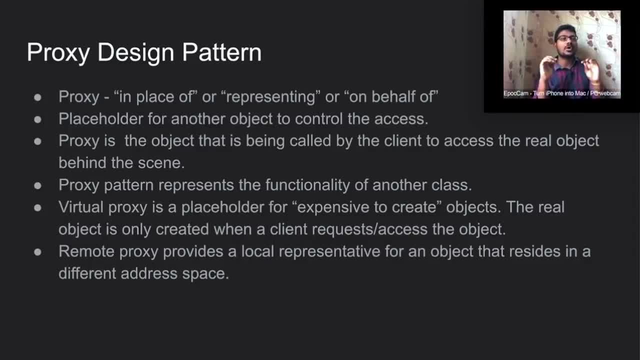 aware about those things. the client knows there will be some object that will be served when we raise a request. so here the proxy object would handle those things. the proxy orbit would get the object from the, from the better address spaces for the particular request. and then protective, proxy, protective. 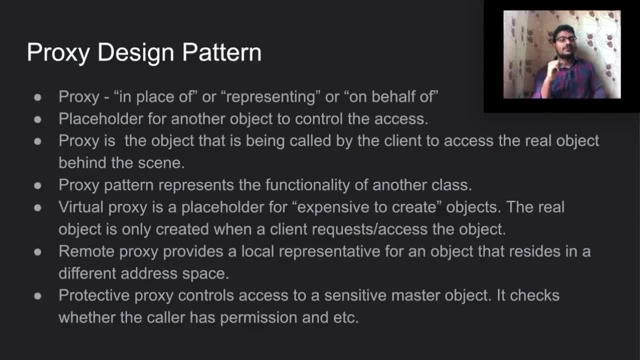 proxy controls, access to a sensitive master object, for example. i have already explained about this example example in the previous video. if suppose, if you're studying in college or some other institutions, you would have some lab session and during those lab session you can access the internet. if suppose, if you are trying to access social web, setting social website, facebook, whatsapp, like that- 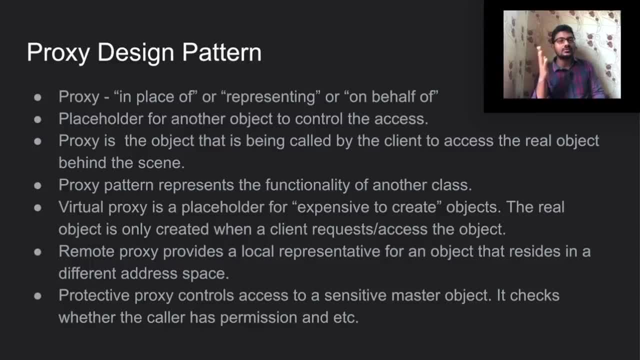 using your college or your institution network internet, then there will be some proxy server which would be, which would be which won't allow you to access the facebook server or whatsapp server. here this is acting as a protective proxy, is protecting the actual request based on the various criteria. 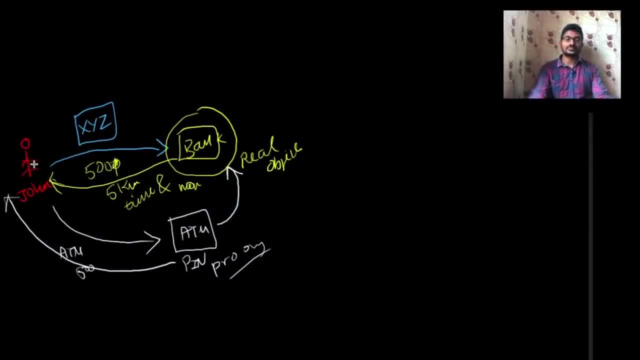 so we will try to relate this with the real life example. this is best example, according to me, for explaining the proxy design pattern using real life example. for example, consider there is a person named named john. he is trying to get 500 rupees from his account, so he is having an account in xyz bank. so what he'd do is he would have 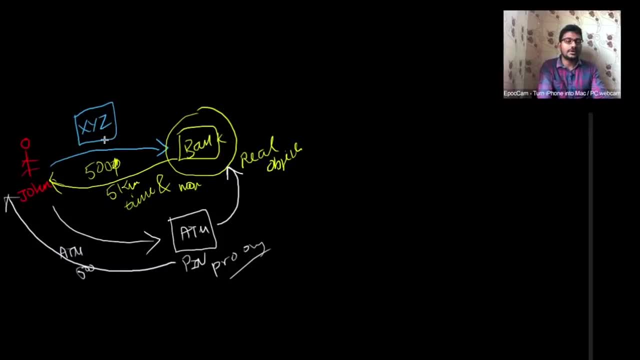 options to withdraw 500 rupees from bank. the first approach is visiting the bank. this is the first approach. in the first approach, what you do is you would try to visit the bank and then you would fill the chalan, withdraw chalan and you will try to and vote that withdraw chalan to the cashier and that cashier would check. 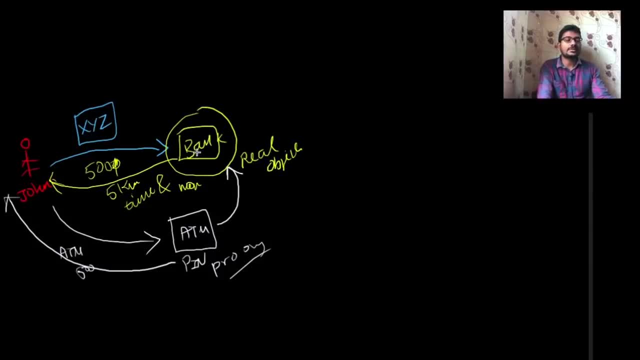 the credentials, whether the account number is valid or not, whether the sufficient funds are present or not, like that. after that that cashier would return 500 rupees to shop is the first neighborhoods. here John is pending money as well as time for withdrawing 500 pieces, for example. consider John is 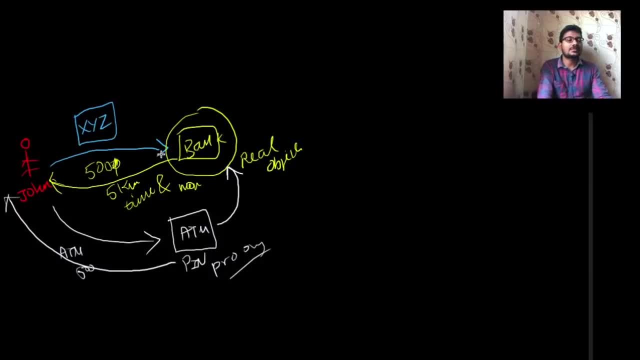 residing at a location. a bank is residing at location B. the distance between A and B is 5 kilometers. for to cover those, to cover the five Kramis John is travelling using bike, so for that he needs to fill some amount of petrol for ú t in. 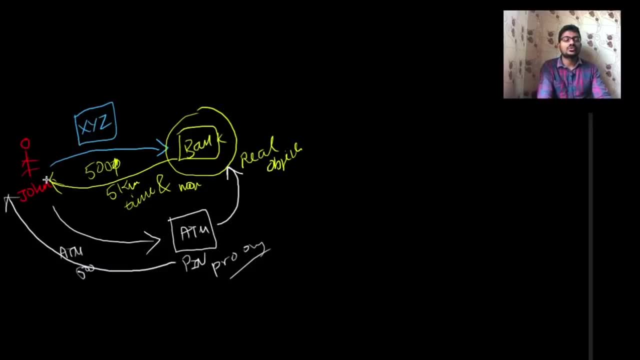 in In to spend some amount of money and then time. so to travel five kilometer it would take some time. so by using the first approach, john is spending both money and time for withdrawing 500 rupees. this is the second approach. this is the second approach where john visits the nearest atm. 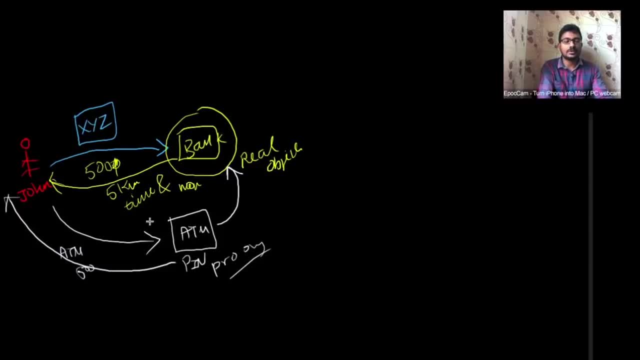 and then he uses the bank debit card- uh debit card- and the swipes that debit card in the atm machine and he enters the required credentials like pin number and other stuff and is entering the 500 rupees in the withdrawal category. here that the atm machine will act as a proxy object. 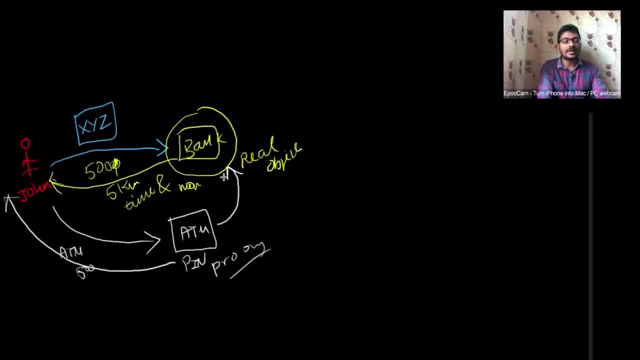 it will try to communicate with the real object called bank and it will check whether that account has sufficient balance and that and and it will check the other credentials and the bank real object will reply those information to the actual proxy object and that proxy object would serve to the uh, would serve the data to john here. 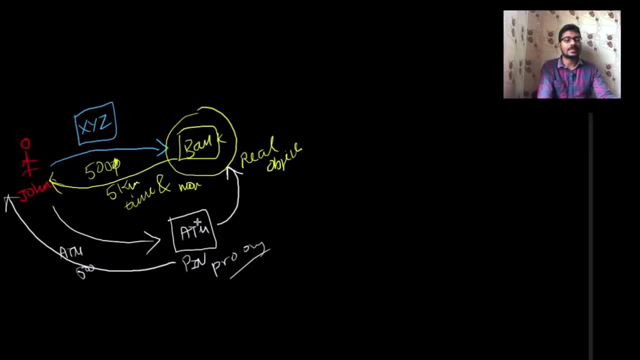 the proxy object is playing the major role, being the screen, this proxy object is handling the request on behalf of us. so by following the second approach, john is saving both time and money, because nowadays atm is present on every street, so he could save both money and time to withdraw. 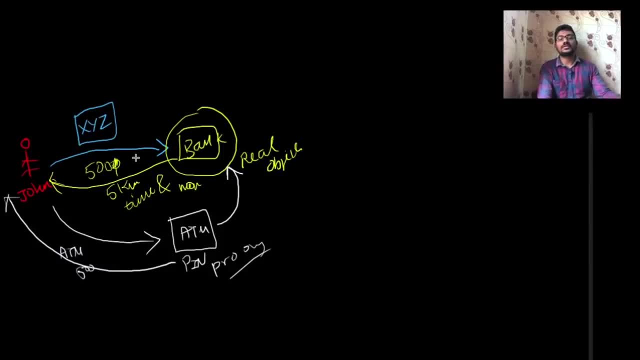 500 rupees. so in real life we are using the proxy design pattern at every point of our life. in software applications also, we are using- we are following- proxy design pattern for some use cases. so you need to first analyze the use case and you need to check whether that 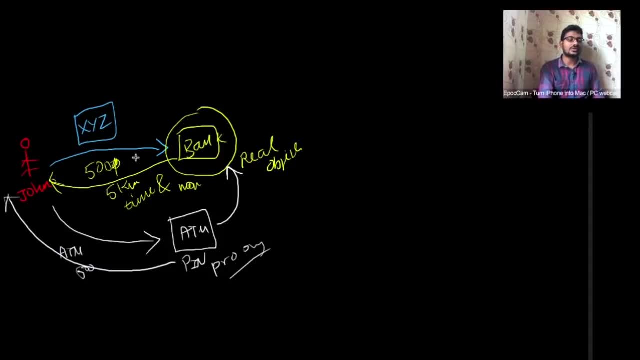 use case could be for could be fit with the proxy design pattern. analyze it. so these are the things about the proxy design pattern. if suppose if you want to learn more things about the software design pattern then you could buy software design pattern book. the book link would: be presented in the description box of this video. so thanks for watching this video.